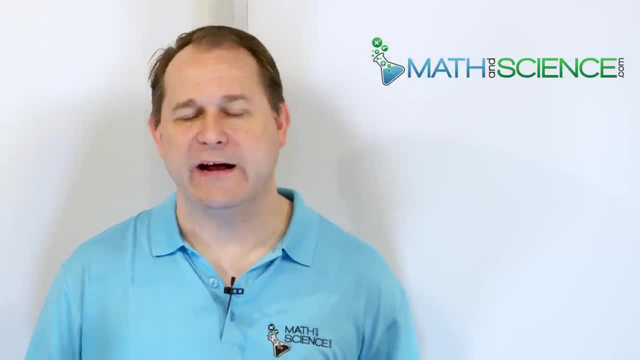 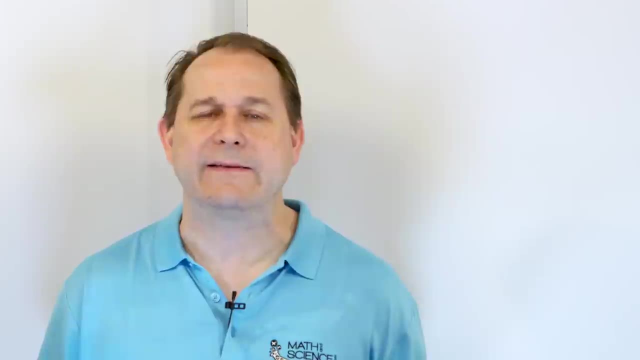 right, That's the big picture. We're going to get into why and what it is in just a second. That's goal number one. Goal number two is I'd like to solve some problems, to give you practical experience using the law of cosines. You'll find out that it's pretty easy to use once you know. 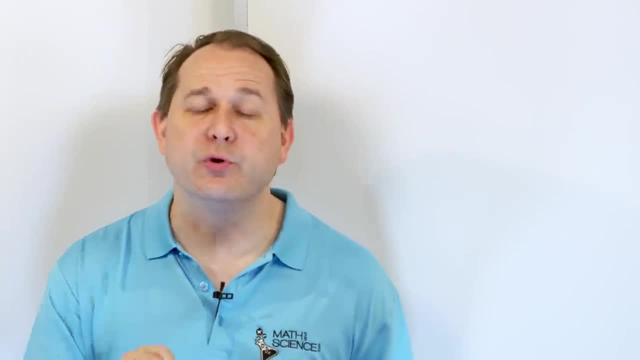 what you're doing. And number three: at the end of the lesson, I'm going to prove the law of cosines to you. So not only will you know what it is and what it's for and how to use it, but by the 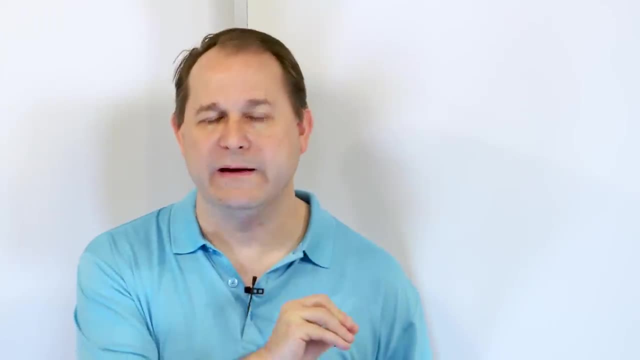 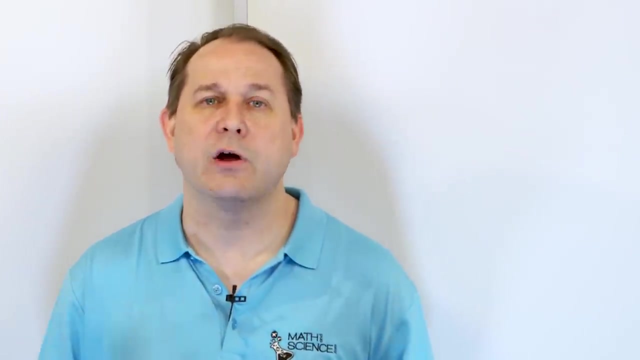 end of the lesson, you'll know exactly where it comes from. You'll know how to prove it And the proof of it. usually I don't do too many proofs, or not, I don't do proofs for everything, But in this case the proof of the law of cosines is really useful because you learn where it comes. 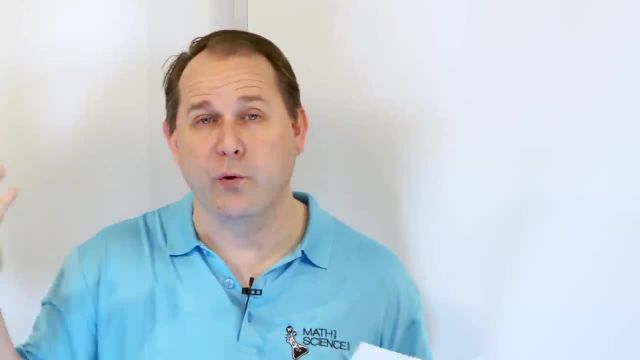 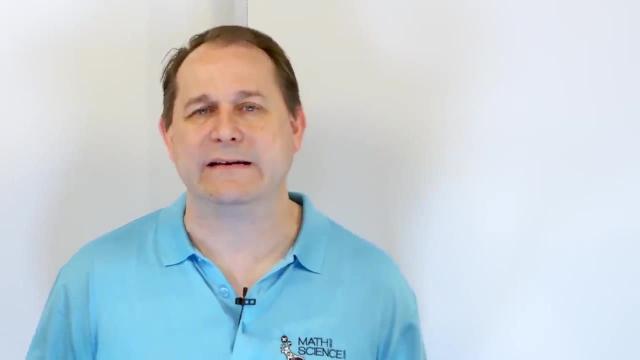 from, but you also the tools that I have to kind of go over With you for the proof. they're actually things that we're going to use later on anyway in math, So they're very useful, And so that's why I feel like it's a good idea to go over that, And so you 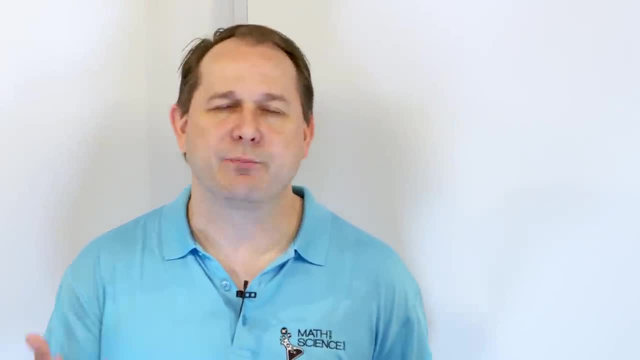 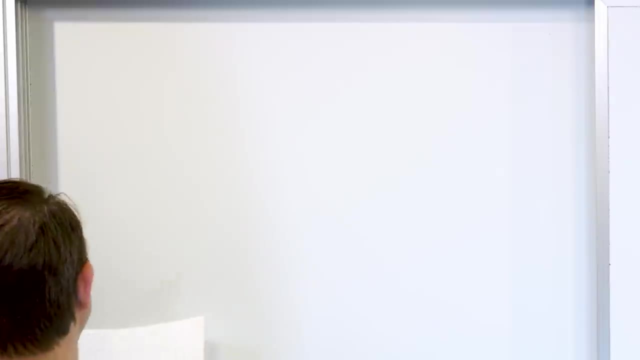 know where it comes from and you get a little practice with the proof, and the proof is not difficult to understand. So I encourage you to stick with me to get there Now. we all know about right triangles. right Right triangles are probably the most useful kind of triangle we have. 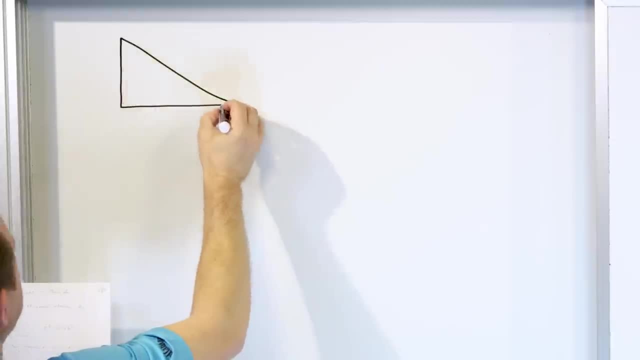 And we can use it for all kinds of problems. right, But just to refresh your memory, here is what a right triangle is. Now, there's a 90 degree angle here and this is going to dovetail into the law of cosines in just. 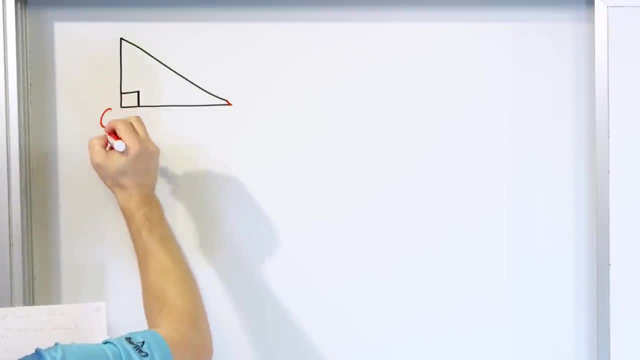 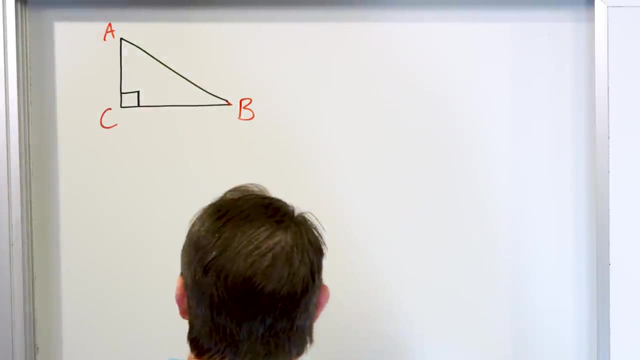 a second. So stick with me here. right, But if we have a angle C right, an angle B, an angle A with the capital letters, then what we do is we say: all right, opposite this angle over here we have. 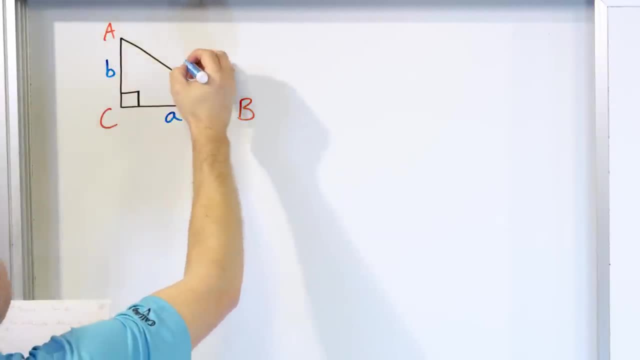 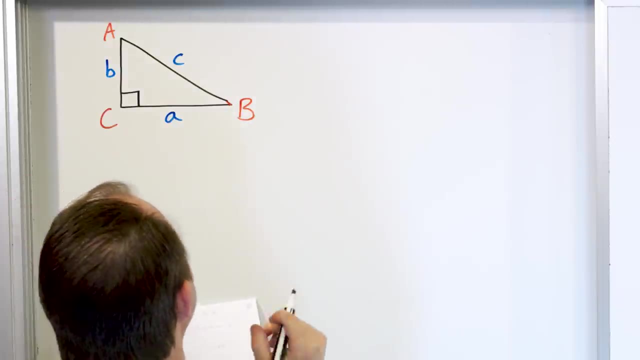 lowercase a. opposite this angle here we have a lowercase b and opposite this angle we have a lowercase c. Now we already know from you know in the past, that we have what we call the famous Pythagorean theorem, which applies to right triangles like this one, And we know that. 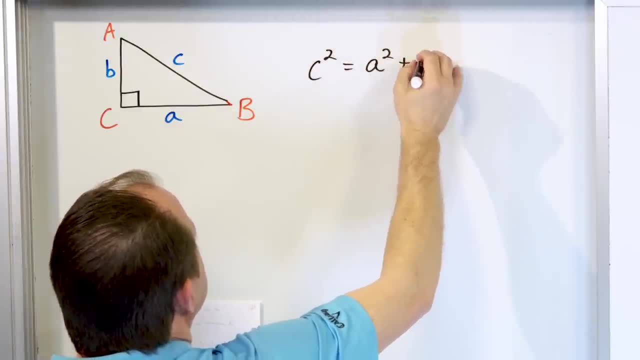 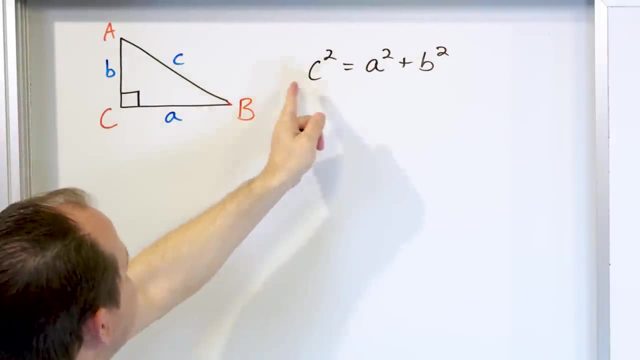 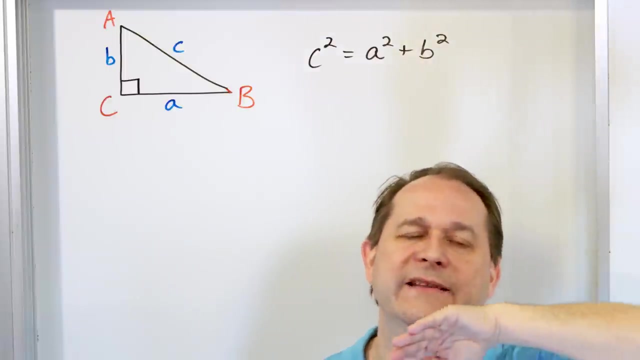 c squared is equal to a squared plus b squared. So if you know it's a right triangle with a 90 degree angle and you know any two of these sides, you can use the Pythagorean theorem to find the value of the third side right. The hypotenuse is always called c and it's the. 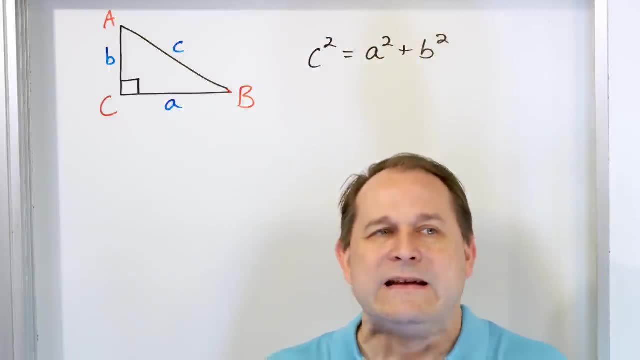 longest side of the triangle opposite 90 degrees. Now it's really useful. but what happens if you have a right triangle? What if you have some other random shaped triangle? Are we just stuck? Do we not have any tools? Well, the answer is: we're not stuck. We have. in this lesson we're going to 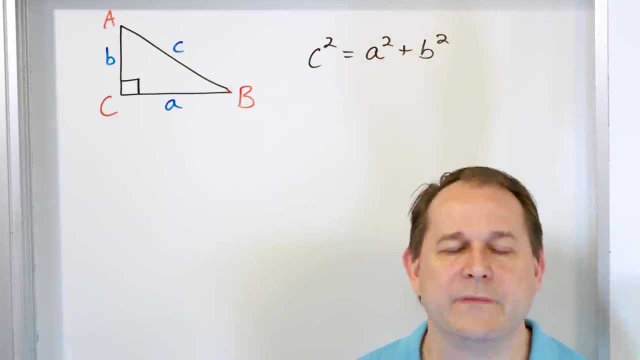 talk about the law of cosines, which applies to any triangle, And then later on we're going to talk about the law of sines, which is a totally separate equation and it's for different situations, but it also applies to all triangles. So for here, let's talk about this law of cosines. 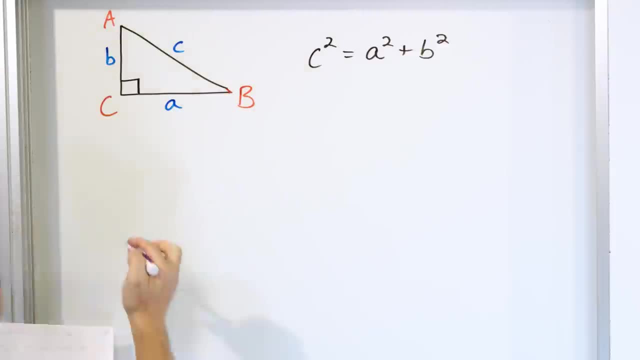 First, without proving anything, we're just going to write it down. So let's go ahead and talk about the situation when we have a general shaped triangle, which is different, And of course this doesn't look like a great triangle because it's got a curved, a little curved line on the 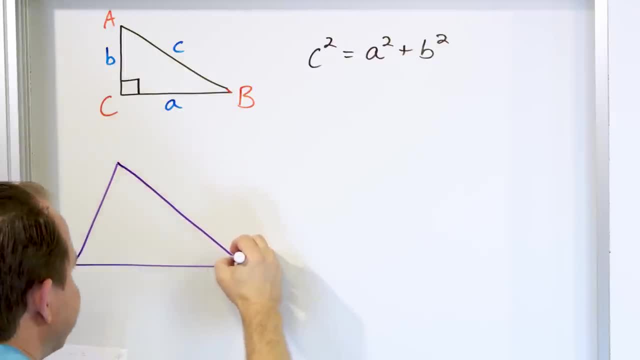 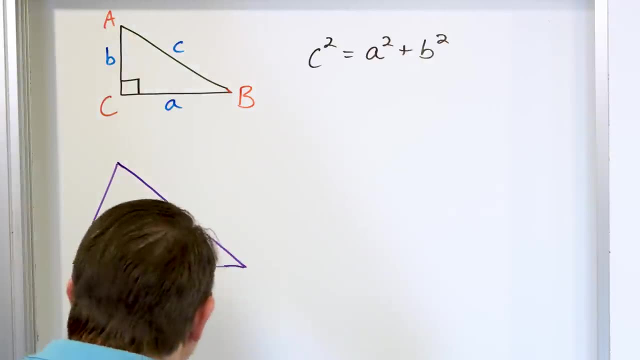 side. So sorry about that, But you get the idea. If I draw a straight line like this and I have a triangle, this is not a right triangle because there is no 90 degree angle in any of these places, But I can do the same kind of thing. right, I can say: this is angle A up here and this I 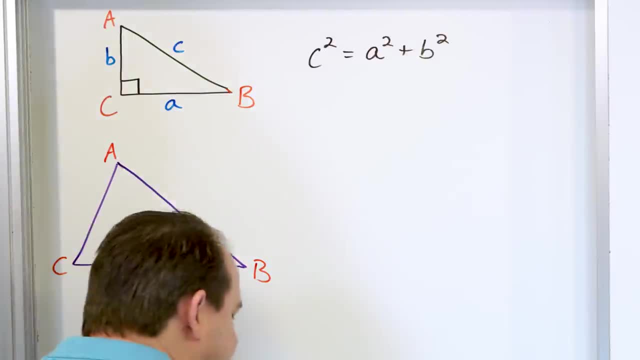 can call angle B and this one over here I can call angle C, And so, opposite of angle A, I can do lowercase a. That's the length of this side. A Opposite angle B, I can call it lowercase b. 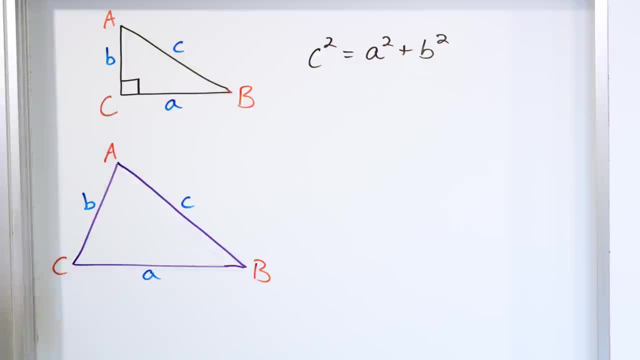 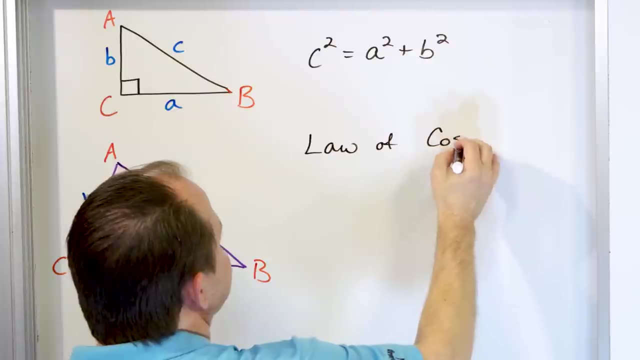 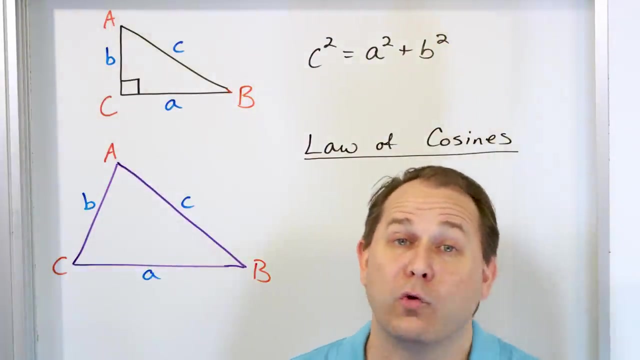 Opposite angle C. I can do lowercase c like this. So I have A, B and C. Now what the law of cosines says, law of cosines is what it does is it is a modified form of the Pythagorean theorem. So you're going to see. 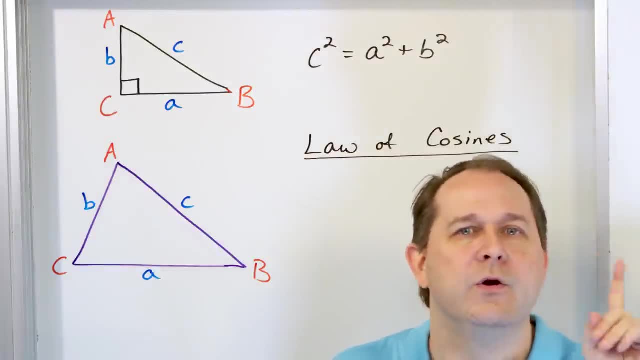 similarities. It's going to look like the Pythagorean theorem, with an additional thing at the end of it which changes it a little bit. It's going to look like the Pythagorean theorem, which changes it a little bit. It's going to look like the Pythagorean theorem, which changes it a little bit. 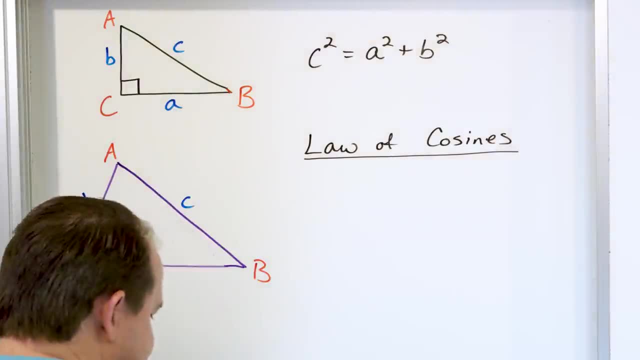 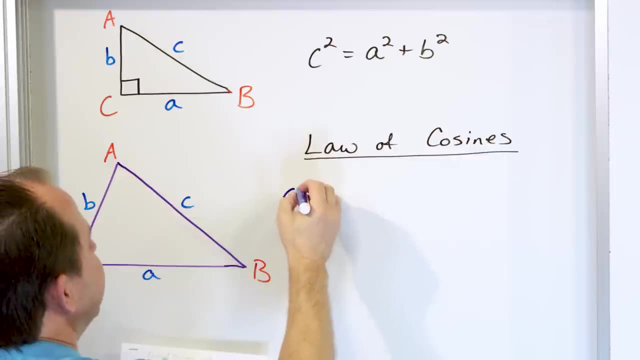 It's going to look like the Pythagorean theorem, which changes it a little bit Because it's not a right triangle. So let me show you what that is. Let's do it in blue. The law of cosines, for the first way we're going to write it is the following: C squared is equal to A squared. 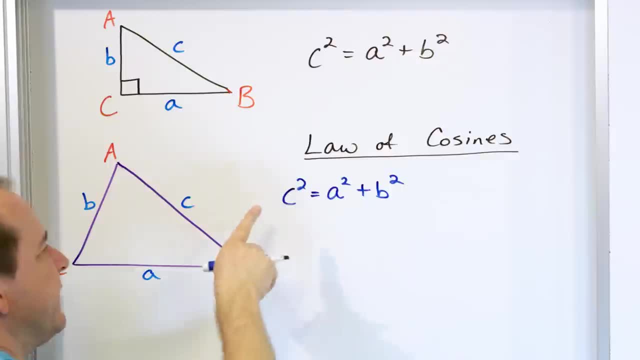 plus B squared, And you're like, wait a minute, That's exactly what we have here. Yes, it's the Pythagorean theorem, with one more thing at the end. So the length of this side C is equal to A squared plus B squared, But then we have minus 2 times B squared. 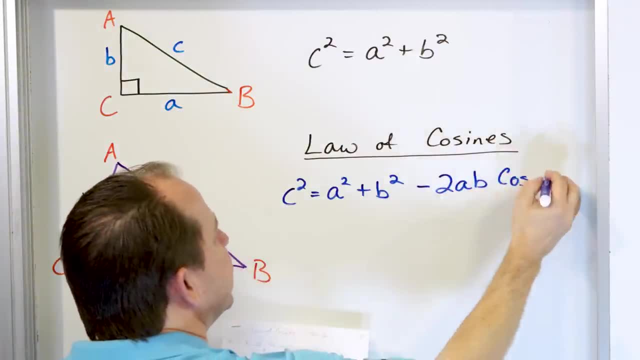 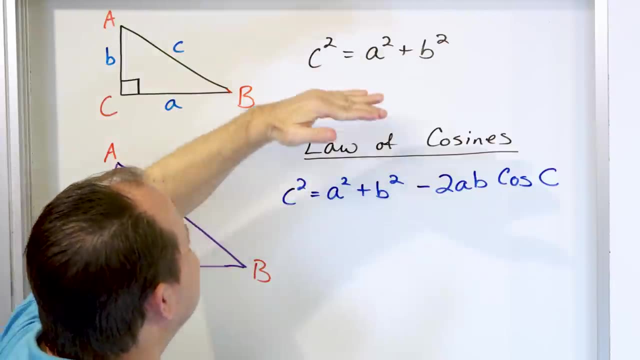 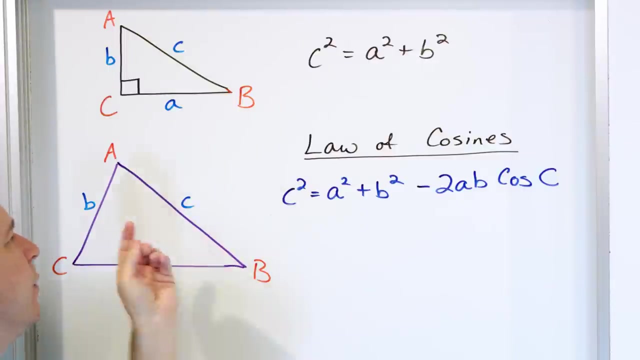 So that's the angle C. So first, before you even talk about it, just convince yourself that this looks exactly like the Pythagorean theorem with one additional subtracted term at the end. So it's because it's not a 90 degree angle here, causing a right triangle, that this causes us. 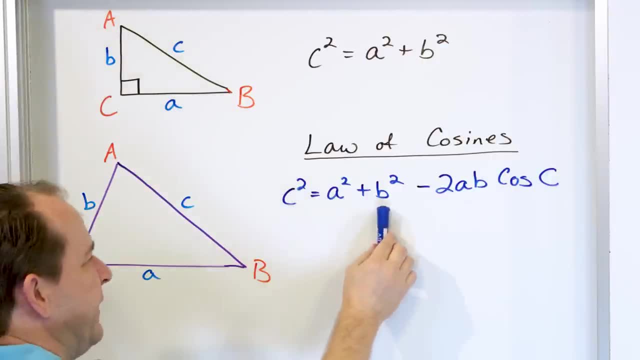 to have to have this extra term. So it's A squared plus B squared minus 2 times whatever you have here, AB, And notice that A and B are right here on the triangle And we have cosine of C here, which is the angle between A and B. So the way it works is: it's the 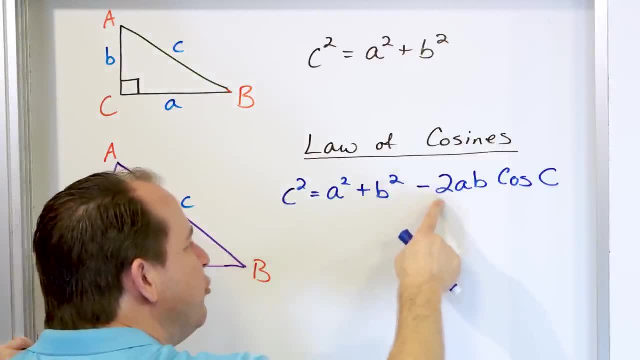 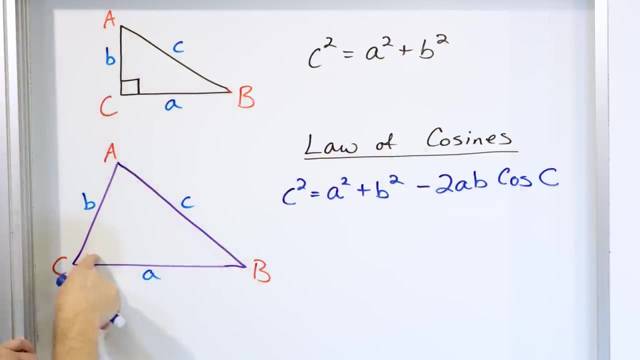 Pythagorean theorem: C squared is A squared plus B squared minus. two times the lengths of these two sides that we have written here times the cosine of the angle that is between them. That's why it's called the law of cosines, because we have this cosine here. Now. this is, if you're trying to. 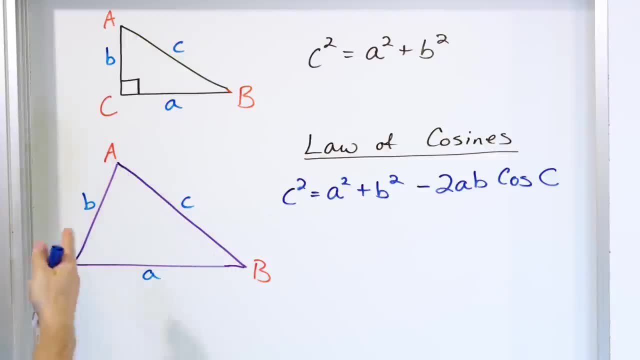 really find the length of side C here. But we can write this law of cosines for the other sides as well. Let's try this. So let's say A is equal to C squared, And then we have the angle between A and B. 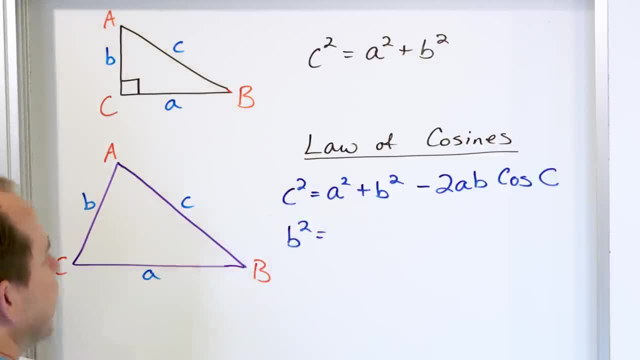 Let's see how the pattern unfolds. B squared is the length of this side. squared is going to be the other two sides squared: a squared plus c squared right, Because if we have one letter over here, the other two letters exist on the other side. 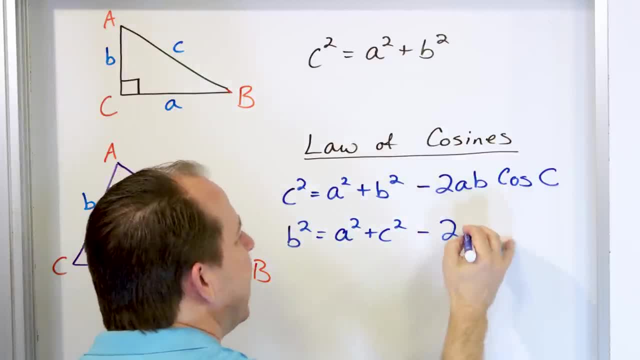 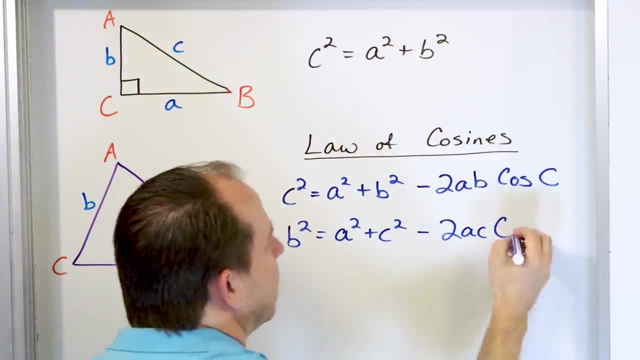 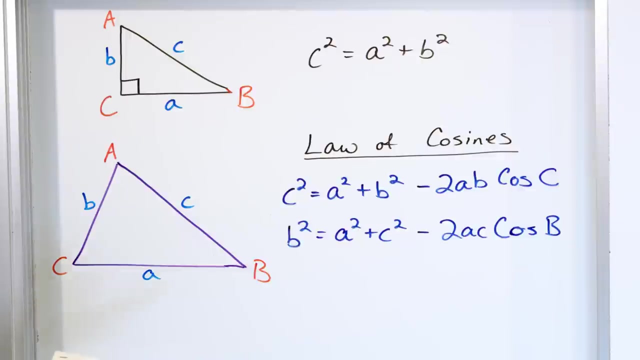 But then we have to have minus 2 times these letters, a times c times the cosine of here's a and c. the angle between, The angle between, is angle b, cosine of angle b. So b squared is a squared plus c squared minus 2a times. 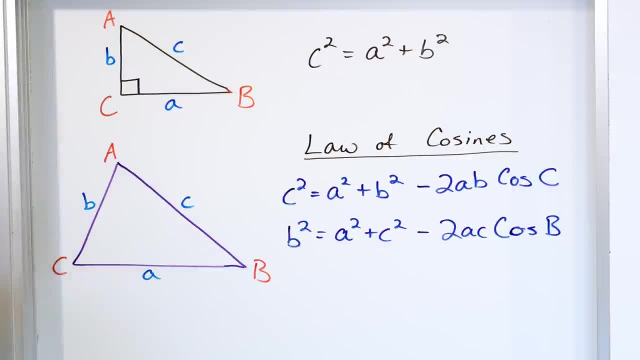 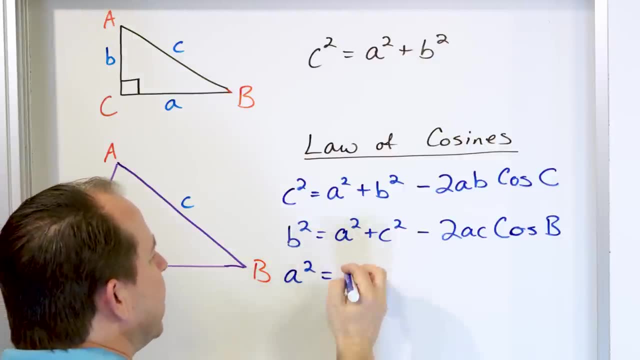 a squared plus c squared minus 2ac times cosine of b. Now let me write the third one down and we'll talk about it again. What if we want to find side a, a squared, Then it's going to be the other two sides squared. 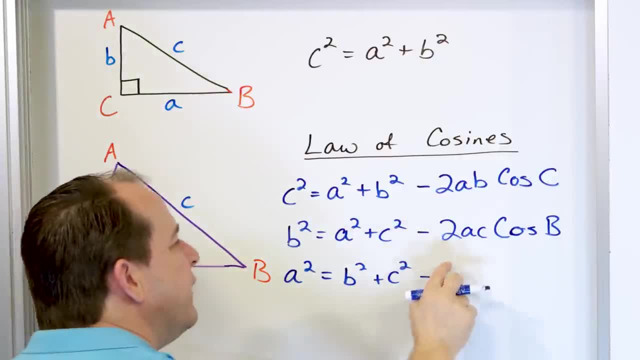 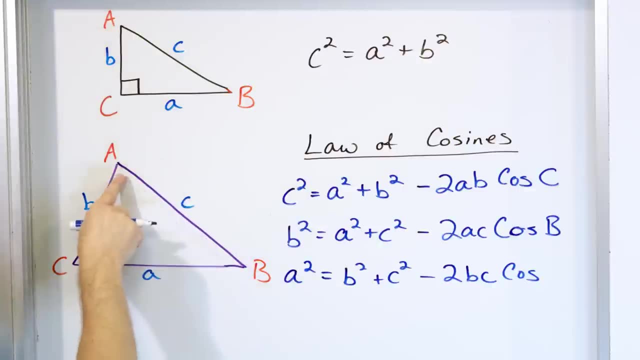 b squared plus c squared. But then I got to subtract 2 times these two sides, b times c times the cosine. here's b and c of the angle between which is angle a. So this is how I want you to remember the law of cosines. 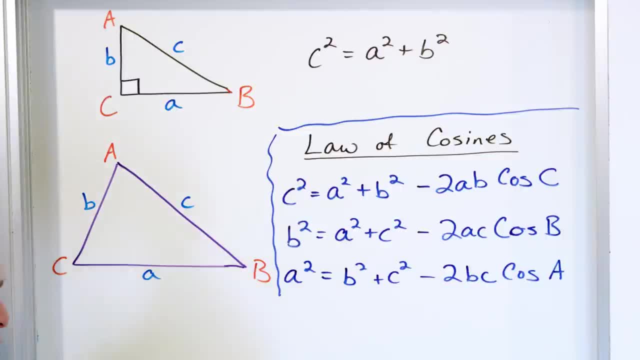 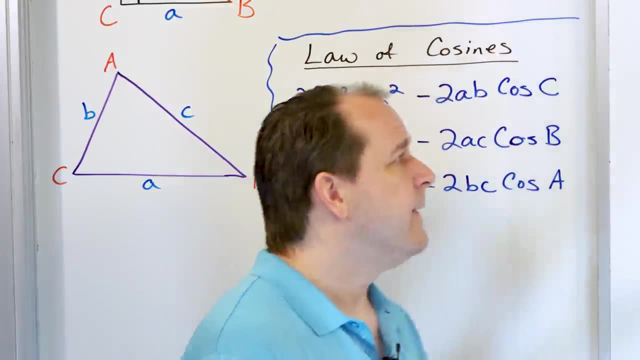 A lot of students just try to memorize them and they don't know, like they don't know what they're really. they don't really see the pattern. So they're just trying to memorize three completely separate equations without understanding the pattern. 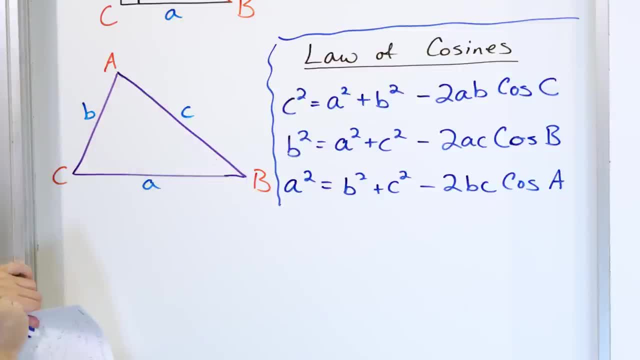 The pattern is in a general triangle without any 90 degree angle. Then the length of one side squared is just the other two sides squared added together. So in this case a and b squared added together minus 2 times these same two sides. 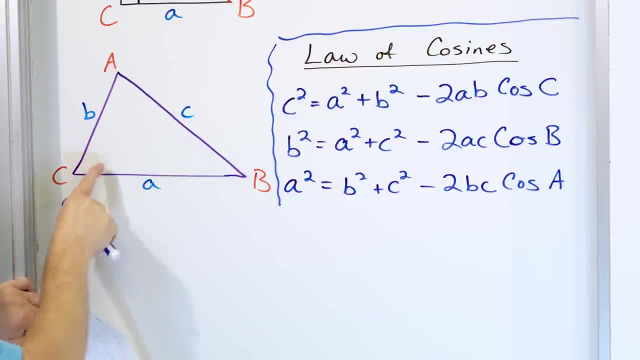 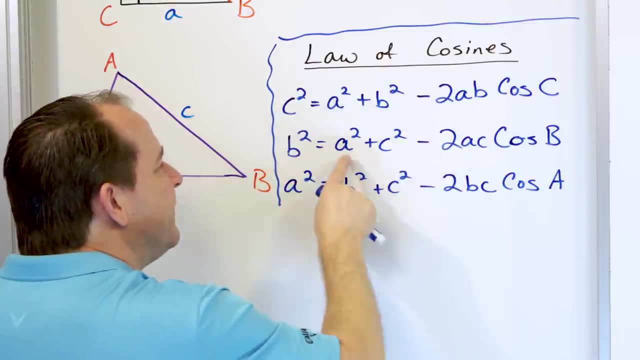 times the cosine of the angle between, In this case between a and b, is the angle c. That's the first equation. If we're trying to find b, it's the other two sides squared minus 2 times these multiplied a times c. 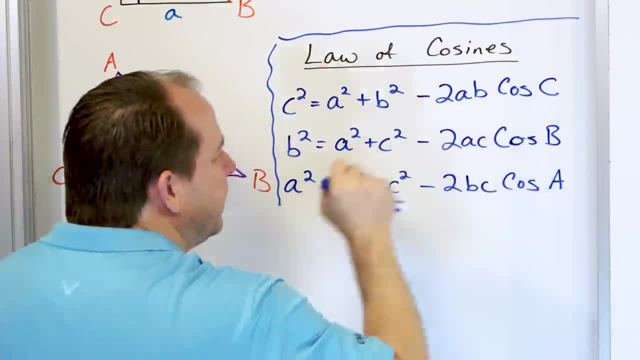 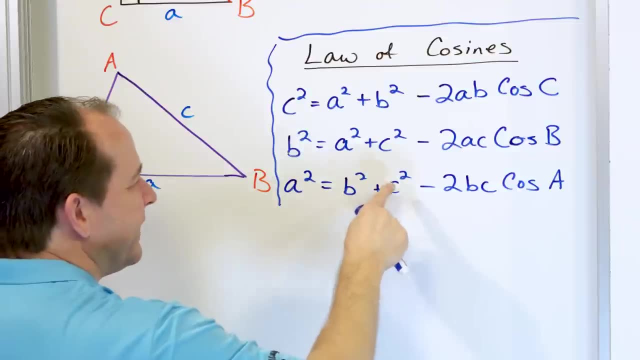 and then a times c. the cosine of the angle between is cosine angle b. And finally, if you're trying to find the length of the side a squared, it's the other two sides squared: b squared plus c squared minus 2 times the same two sides, bc. 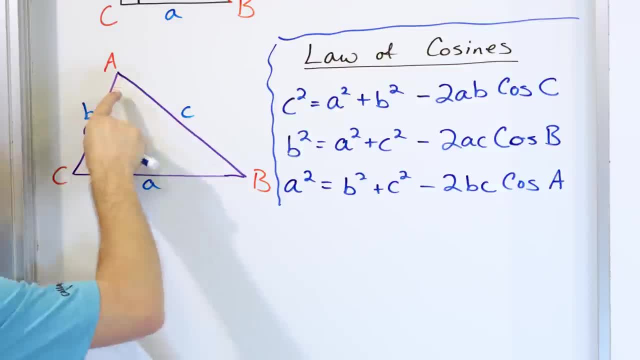 times the cosine here's b and c of a, which is the angle between them, And these are the law of cosines written for whatever side you're trying to find, either A or B or C. Now they're squared. so once you calculate the right side, you'll have to take the square root to get these A, B and C. but that's what it is. 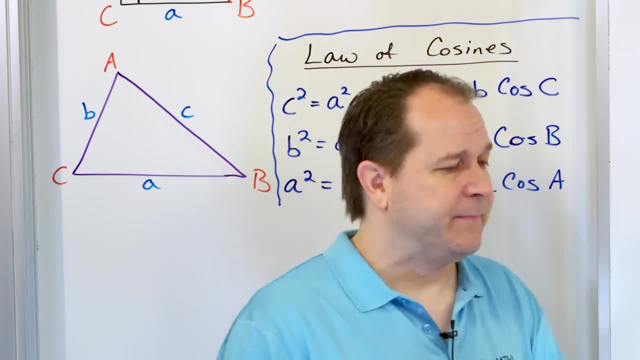 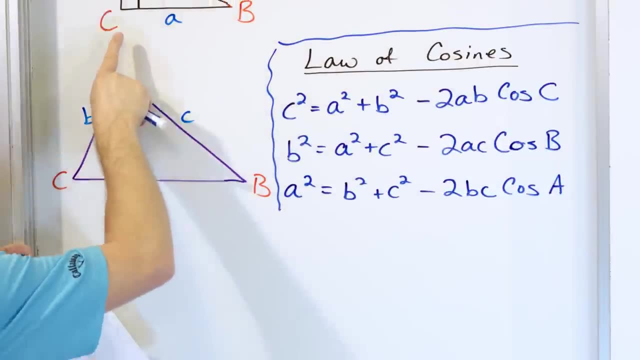 Now let's back up the truck a little bit and cover up these bottom two- Just ignore them right there- And let's say: this is a general triangle, right? Notice, the right triangle has a 90 degree on the location of C. 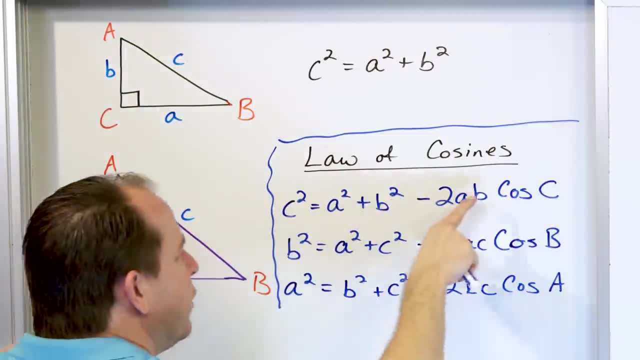 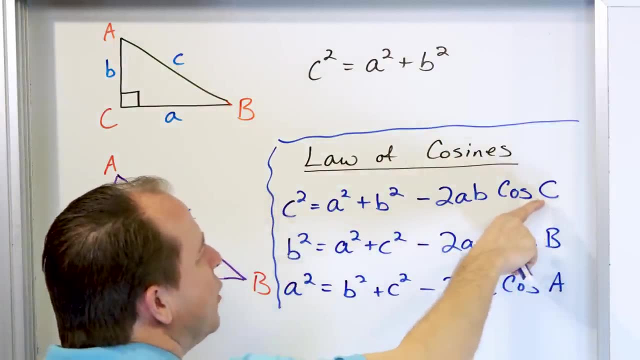 Angle C is 90 degrees. in this case, What if we take the law of cosines right here? and what if we make angle C 90 degrees? In other words, let's put a 90 degree angle in here. What is cosine of 90 degrees? 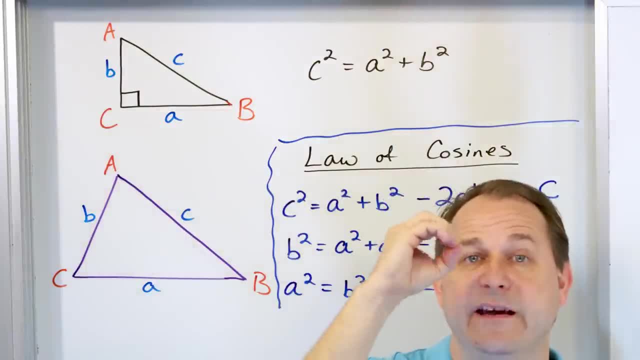 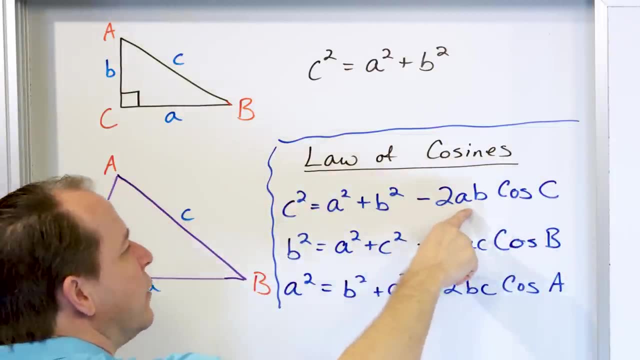 Well, if you think back to trig, cosine of 90 degrees is zero. So if you put 90 degrees in for this angle, you get cosine of zero, which is zero, which kills this whole term. And in the case of a 90 degree angle, here C squared is A squared plus B squared, and all of this disappears. 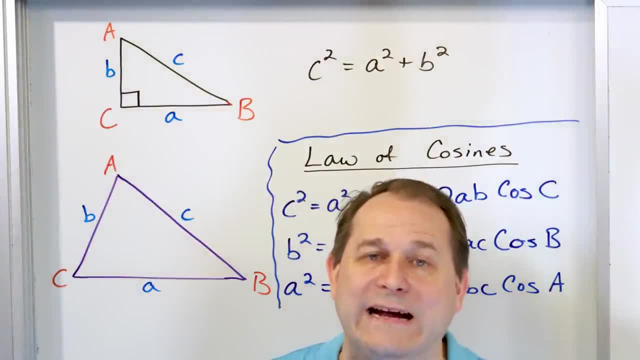 So in the case that you make, If you make one of the angles 90 degrees, you get the Pythagorean Theorem back. okay, If you make C- 90 degrees, you get exactly the Pythagorean Theorem back. If you make B- 90 degrees, which would be this angle right here, then you get a different-looking Pythagorean Theorem. 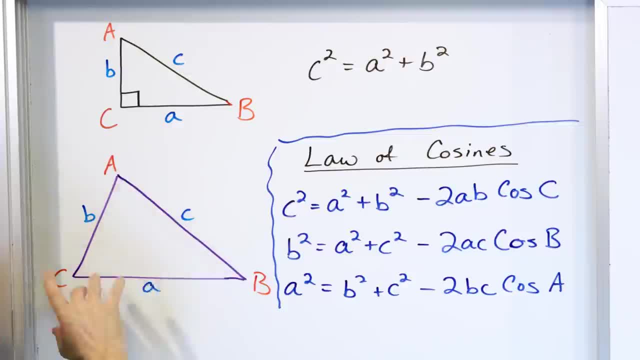 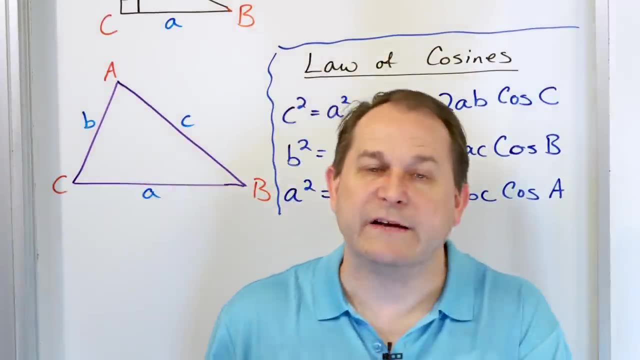 but your 90 degree angle is in a different place, so A and B and C are relabeled. That's why it looks a little different, but it is still the Pythagorean Theorem. So I guess I'm just trying to point out to you that the law of cosines 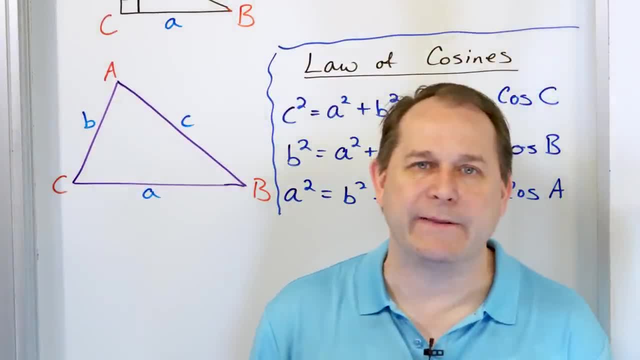 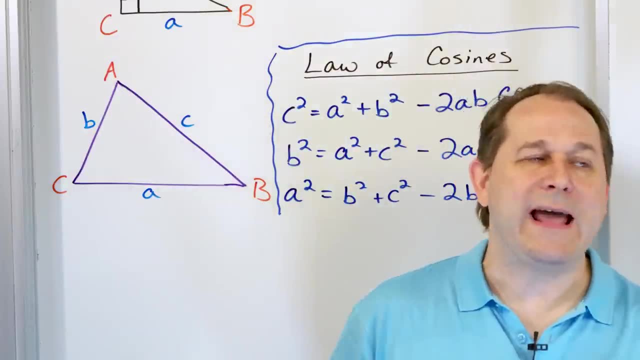 truly is just a modified form of the Pythagorean Theorem. Even if you take one of the angles and make it 90 degrees, then the law of cosines- one of the terms- drops away and you're left with the same Pythagorean Theorem that we learned way back in the beginning. 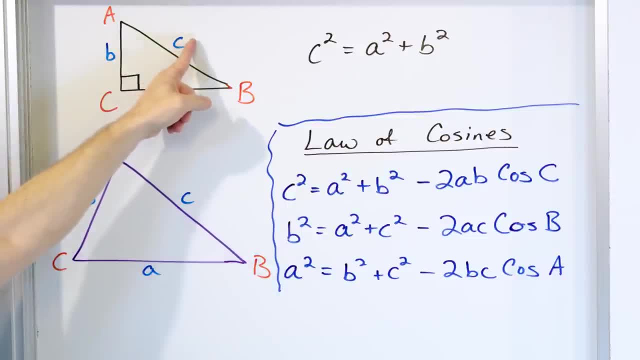 C squared is A squared plus B squared. Notice that C was always the letter opposite of the 90 degree angle. So this is kind of like the prime law of cosines, and the other ones are just written for the other sides. So now that we kind of understand generally what the Pythagorean Theorem is. 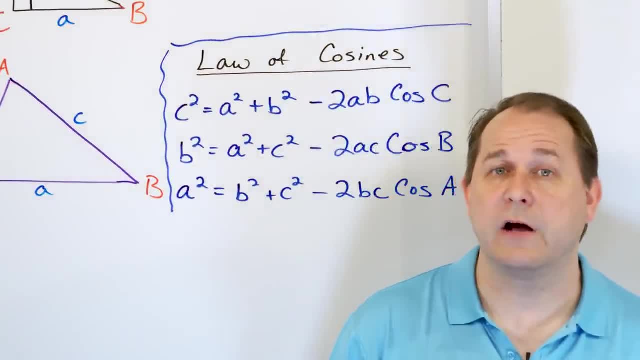 So now that we kind of understand generally what the Pythagorean Theorem is. So now that we kind of understand generally what the Pythagorean Theorem is, let's go ahead and solve a couple of quick problems and then stick with me to the end. 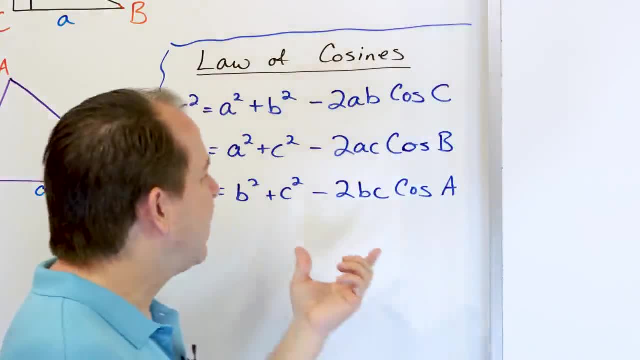 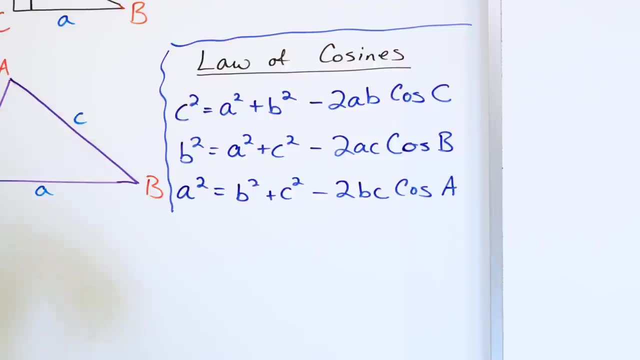 because then we're going to prove this, We're going to start from the beginning and we're going to actually prove that this thing is true, so you know exactly where it comes from. All right, so let's do that, Let's go over here, and I think we can solve the first problem just right underneath here. 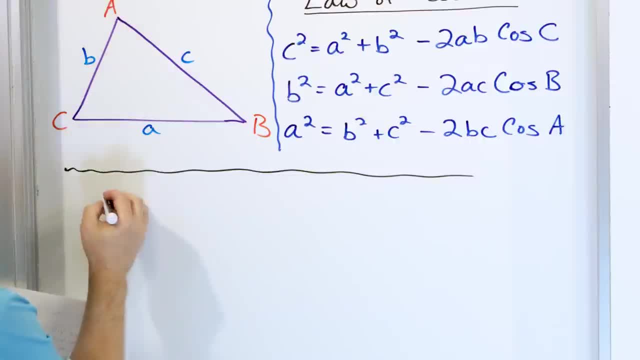 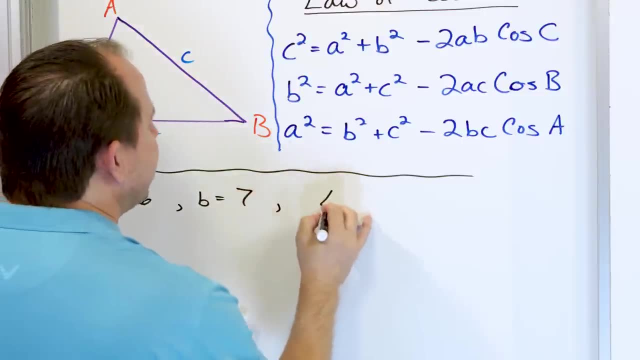 Let's say that I give you that a general triangle- it's not 90 degrees- that the value of A is equal to 6, and the value of side B is equal to 7, and the value of the angle C is equal to 20 degrees. 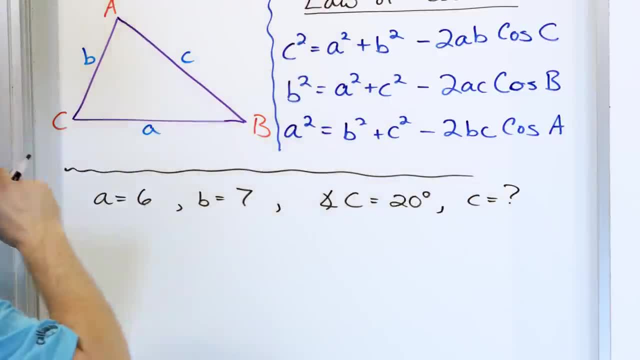 And I want you to tell me. tell me what side C is equal to. So the first step you should always do is draw a picture. So draw a picture. Don't draw a 90 degree triangle, though, because this is not a 90 degree triangle, right. 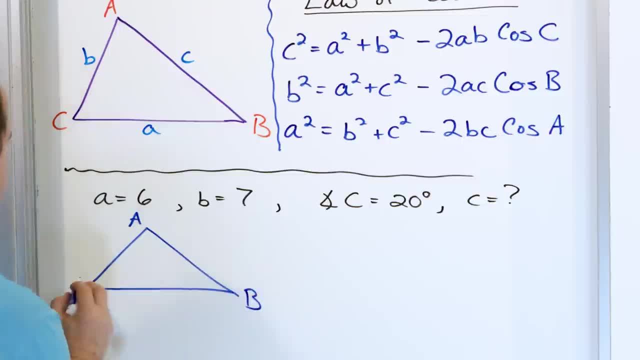 But you have angle A and you have angle B and you have angle C, And then opposite angle A is side A and opposite angle B is side B and opposite angle C is side C. So now that you have these in place, 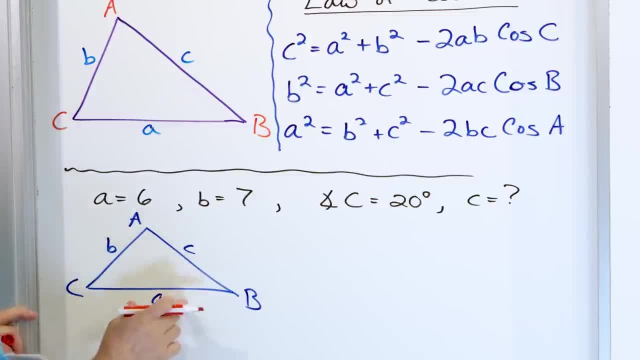 you can actually list or put the measurements on here. So you know, side A is equal to 6, side B, here is, I'll put a equal to 7 right there. Measure of angle C, which is opposite this one here, this one's 20 degrees. 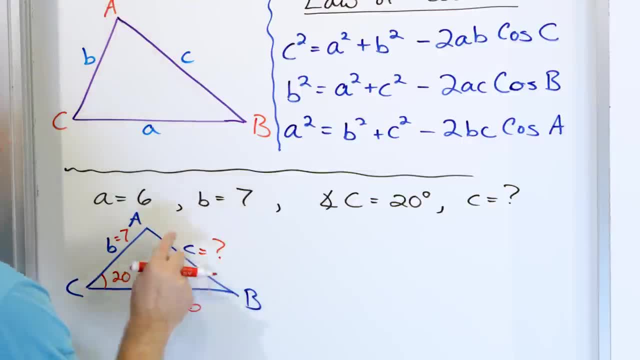 Like this: that's what is here and we're trying to find this one. That's what we're trying to find, side C. So because we're trying to find side C, we look up here and we say, well, we're just going to use the first one, because it's already solved for C squared. 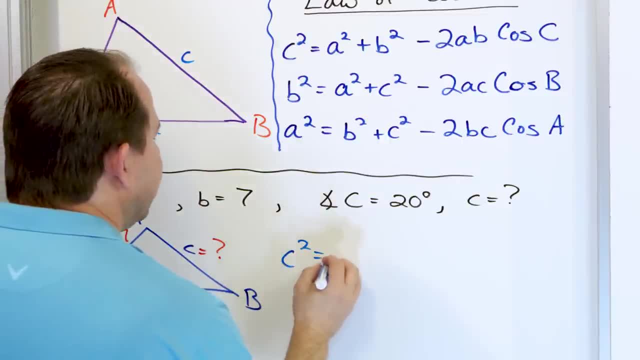 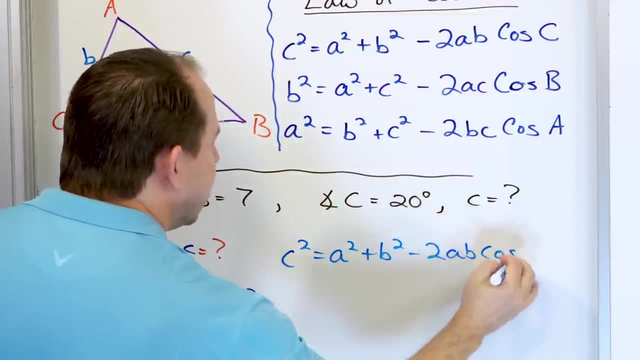 So we're going to write it down And we're going to say that C squared is equal to A squared plus B squared, minus 2 times the same 2, AB times the cosine of the angle between which is the cosine of C, right? 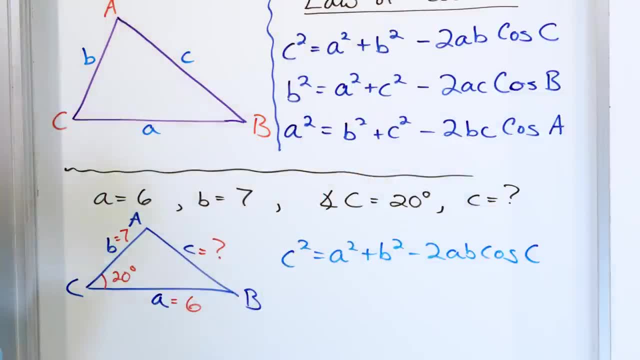 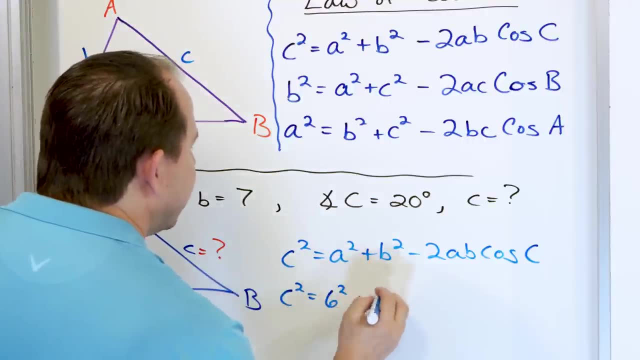 If you don't remember that, then you just copy it down, but I'm trying to also teach you how to remember it. So C squared is equal to A. squared A is 6, so 6 squared plus B squared B is 7, so we'll put 7 squared here. 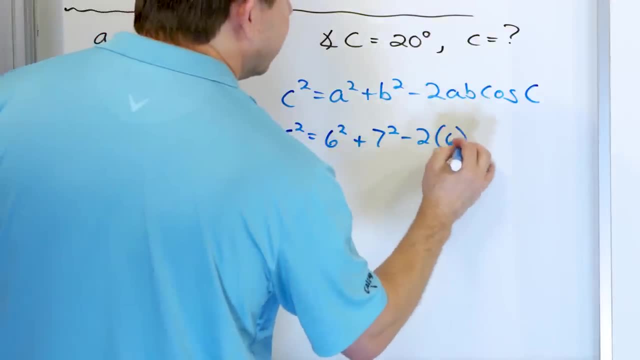 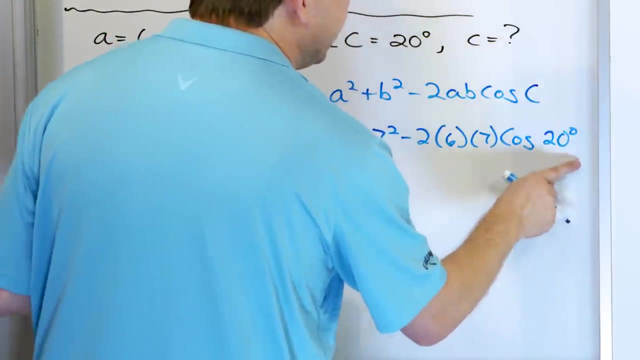 Minus 2 times A, times B, so 6 times 7, times, the cosine of the angle between Angle C is 20 degrees, And you can see that we know all of these numbers, so we can then solve for them. 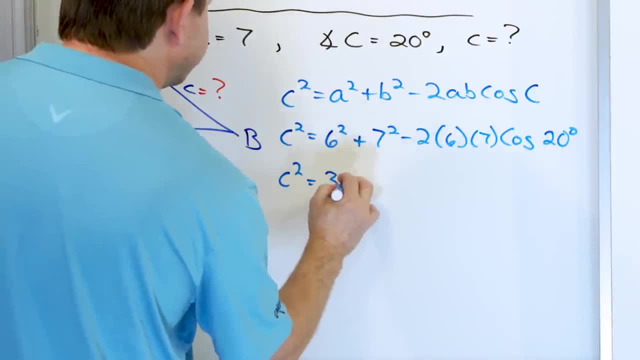 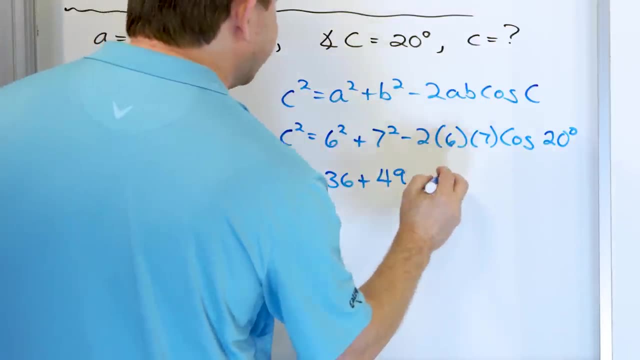 C squared is equal to 6 times 6 is 36.. 7 times 7, 49. And then minus here the 2 times the 6 times the 7 is going to give you 84. And the cosine of 20 degrees. when you put that in the calculator you get 0.9.. 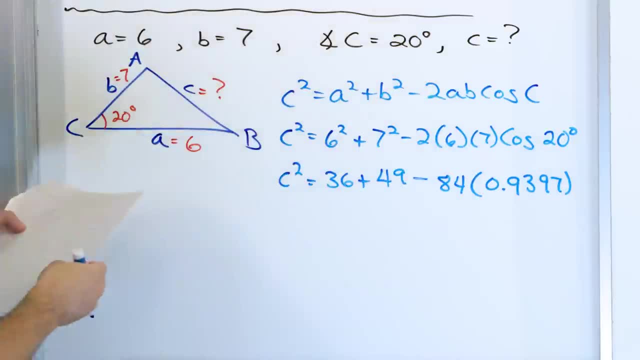 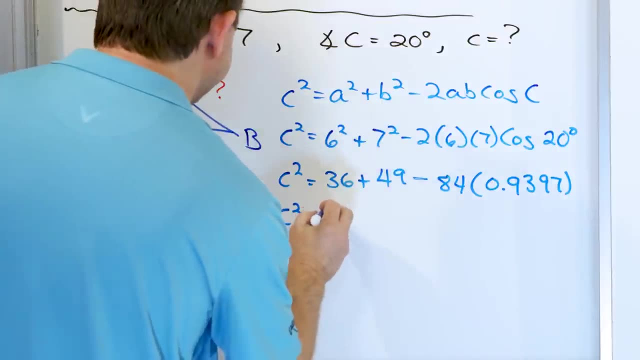 3, 9, 7.. That's the cosine there, And the rest of it is just straight math. So C squared. when you take this plus this and you subtract- well, I guess I'll do these two together- it'll be 85.. 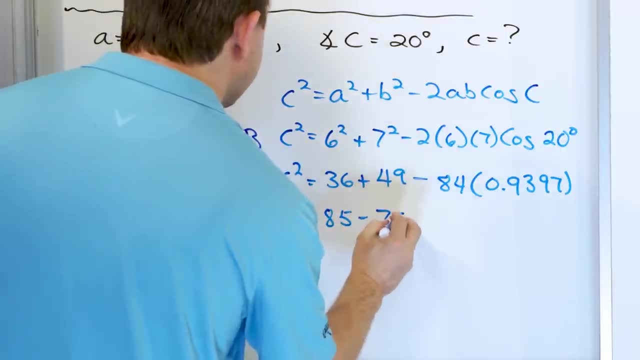 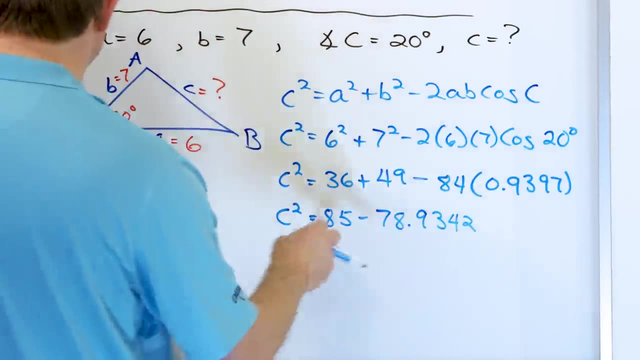 And then this here: when you multiply these two numbers together, you get 78.9342.. And then, C squared, when you take 85 minus this, you get 6.0058.. 6.0058. 6.0058.. 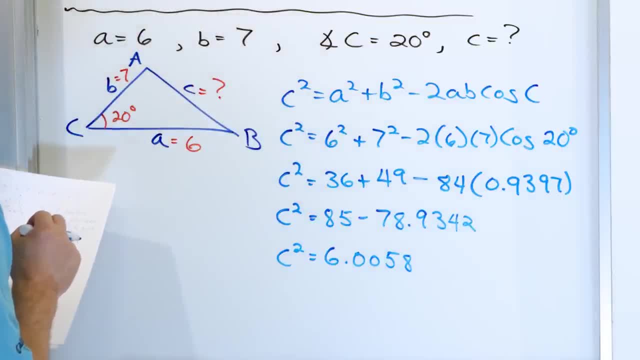 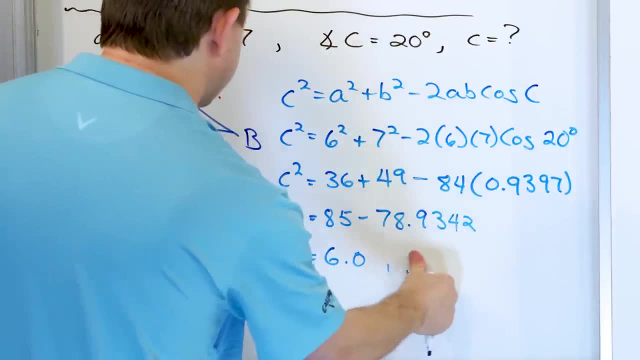 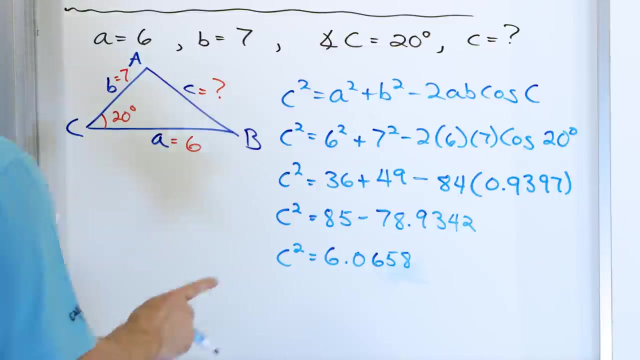 6.0058.. 6.00,. let's see here C squared. no, no, not 0058.. Sorry about that, It is 6.0658.. 6.0658.. Sorry about that. Now to solve for C: see, this is what C squared is equal to. 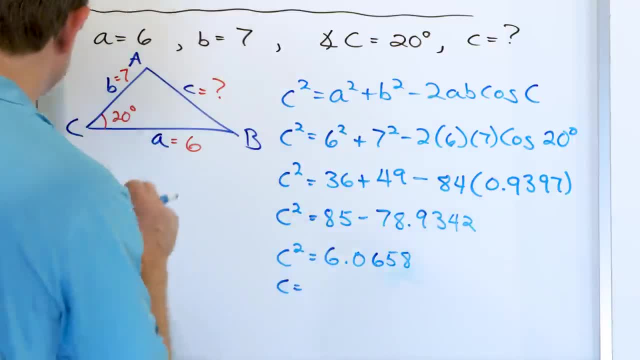 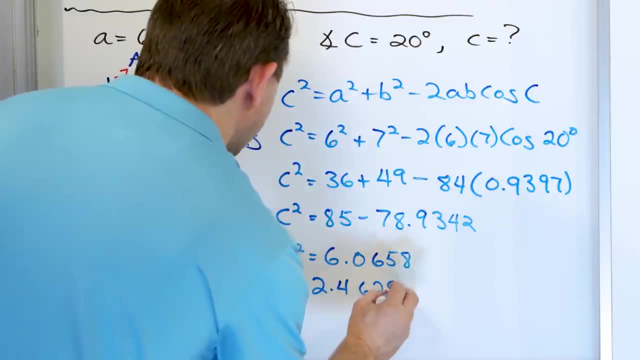 To solve for C, we take the square root of both sides. So the value here of C, when you take the square root, 2.42, or 4629.. Which is approximately equal to 2.46.. So this is what I'm going to circle for the value of C: 2.46.. 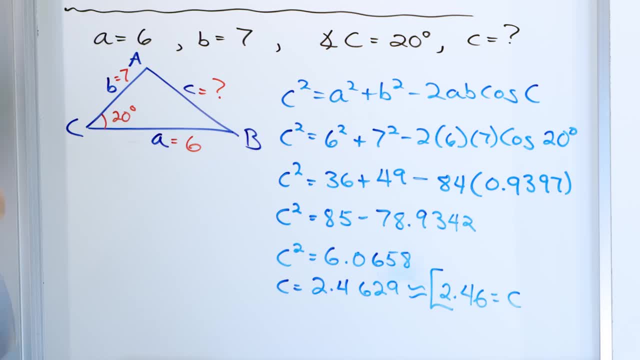 So 2.4629, approximately equal to 2.46.. Now be honest with yourself. Yes, it's a little bit of math, but it's really not that hard. It's literally plugging numbers in and following order of operations. 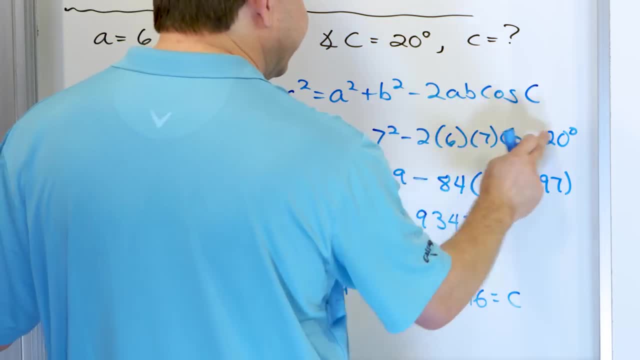 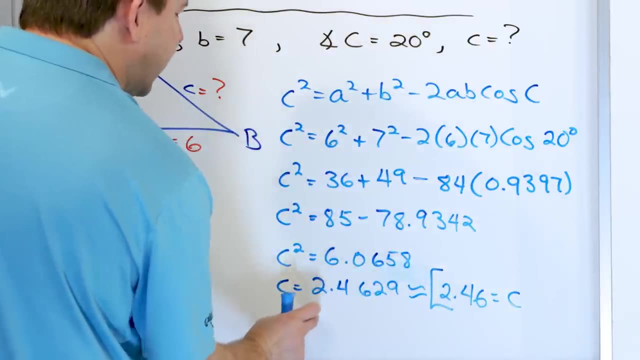 We know we have to square. first We do that and we have to do the multiplication. We do that Cosine is in there and then we have to do left to right addition and subtraction. Once we get the answer, we have to square root both sides to get rid of the square that is over here. 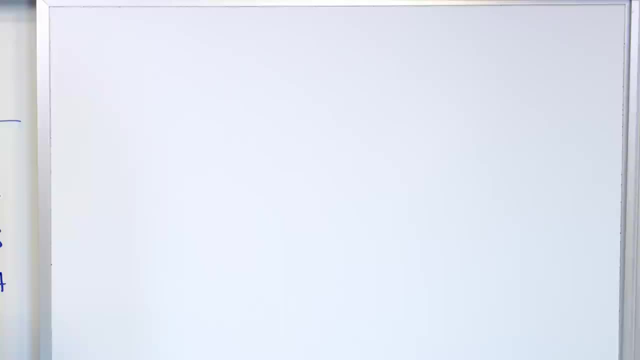 All right, So that's the law of cosines for the first problem. Now let's solve problem number two. Let's say that I tell you that the side C is equal to 15 centimeters, or whatever, And I tell you that side B is equal to 30 centimeters or whatever it is. 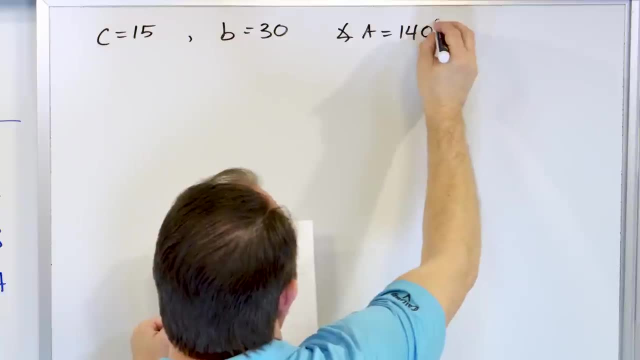 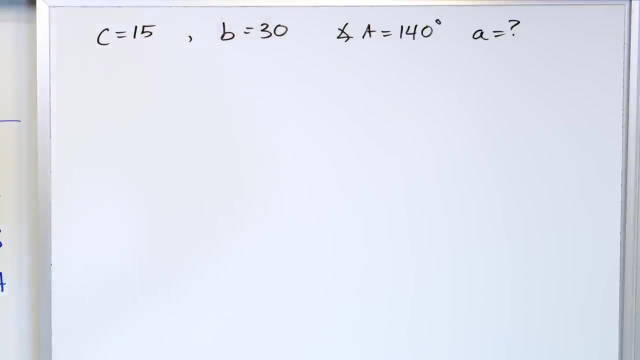 And I tell you, the angle A is equal to 140 degrees. And I ask you, tell me what side A is equal to. Tell me what side A is equal to. So first we always draw a picture. Now, because one of these angles is so big, I'm going to draw the triangle a little differently. 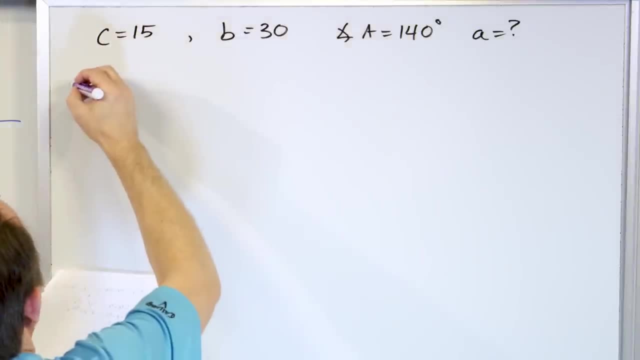 because I know one of these angles is a large open triangle, So I know it's going to look something like this. I mean, I don't really know exactly what it looks like, but I know it has to be open. I'm going to say this is side A or this is angle A. 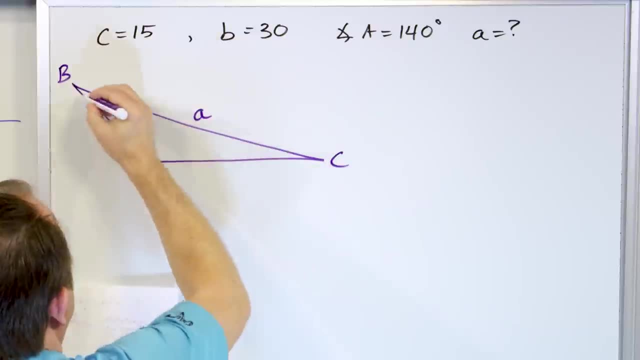 Sorry, this is angle B, This is angle C, And then this will be side A- opposite here, side B, opposite here, side C. Why did I draw it like this? Because then I can draw one of these angles at 140 degrees. 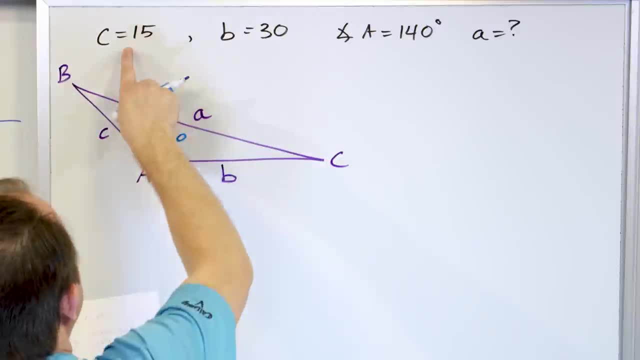 That's very open, Right. And then C was equal to 15.. So that's 15 over here. B was equal to 30. 30 over here. So this is the information I have And I'm trying to find side A. 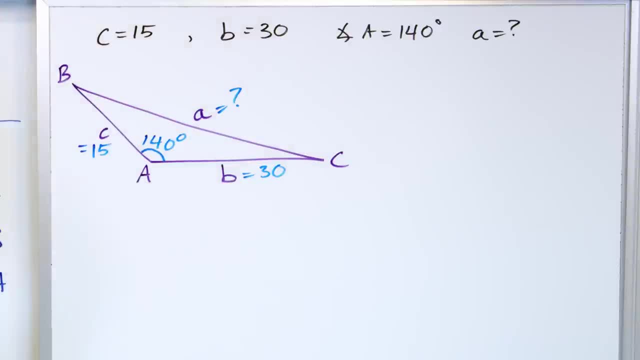 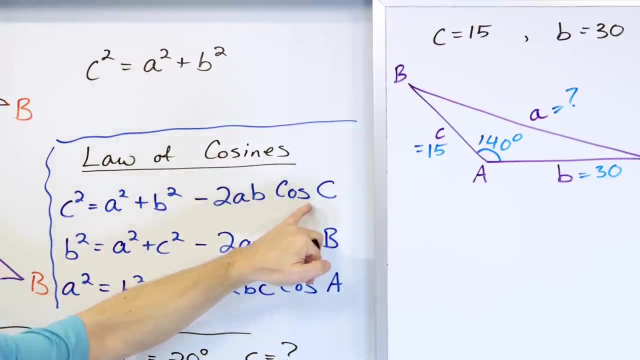 That's what I want to calculate. So let's figure out. what do we want to do? Well, we don't really want to use this law of cosines because we don't even know We need to be able to take the cosine of one of the angles. 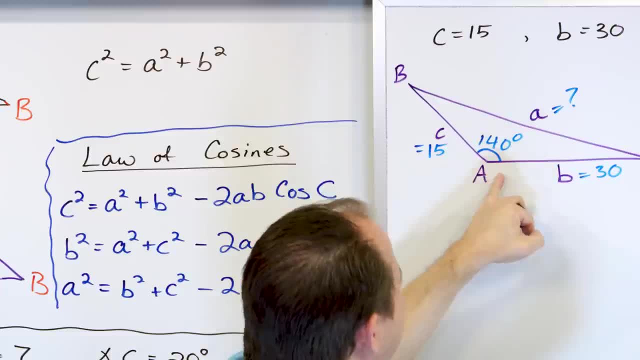 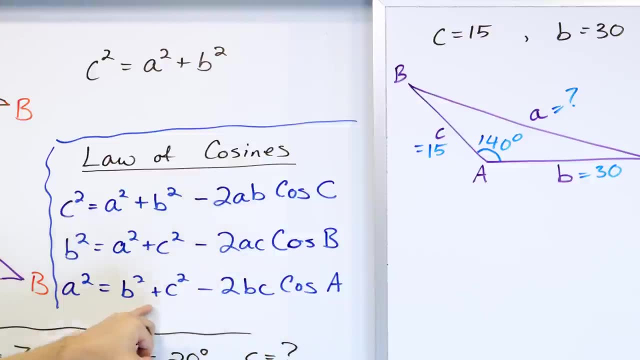 But you see, we only know one of the angles, We only know angle A, We don't know angle B Or angle C. So we want to use the law of cosines that has the cosine of the angle we have And it's also solved for A squared. 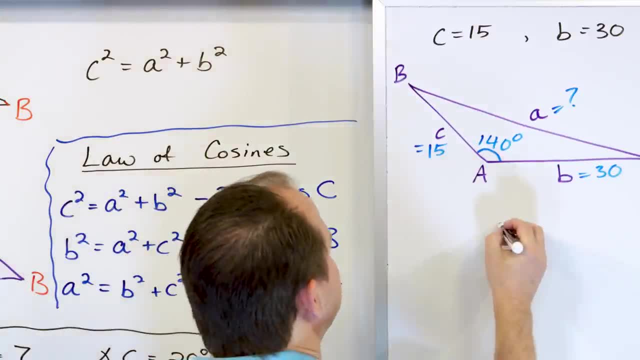 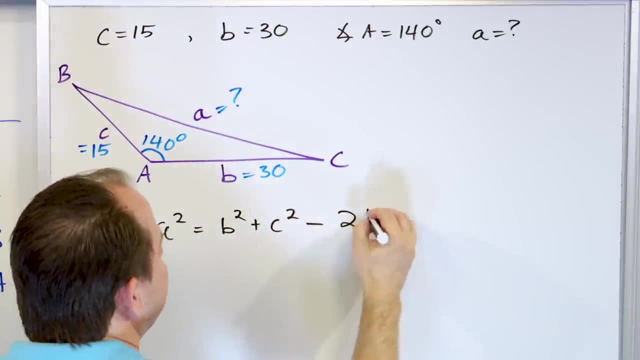 And that's what we're trying to find. So we're going to write this one down. So it's going to be: A squared is equal to the other two, B squared plus C squared minus 2 times. whatever you have here, B times C times the cosine of the other letter. 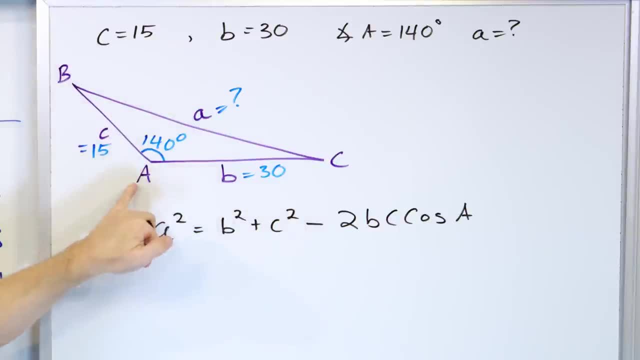 The angle that's between B and C is angle A. So that's what we have: 2BC cosine angle A, All right. So what is side B? That's 30.. So we have 30 squared. What is side C? 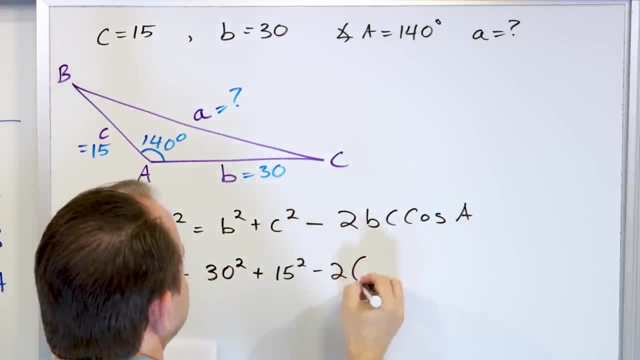 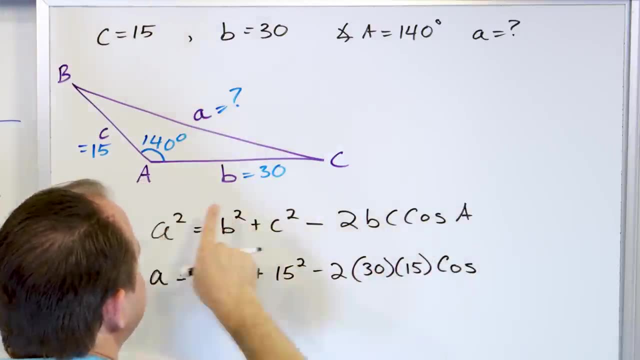 That's 15.. So we have 15 squared minus 2 times BC, which is 30 times 15, times the cosine of the angle between. The angle between is 140 degrees. That's exactly why we use this one, Because that's the only angle we know. 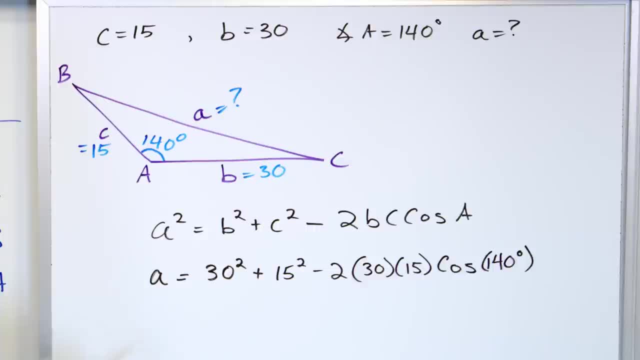 We can take the cosine of that angle. Now, these are all just simply numbers. we can calculate: So 30 times 30.. And this is, by the way, A squared. Sorry about that, Should be A squared. So 30 squared is 900.. 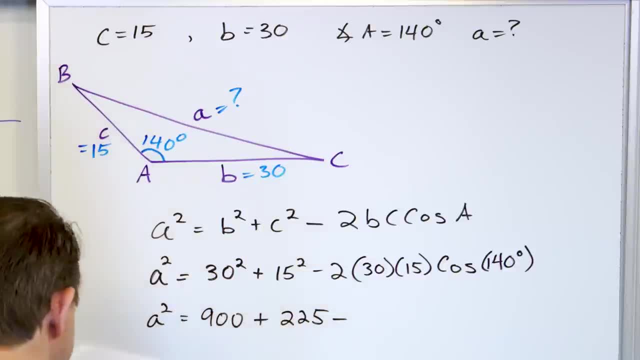 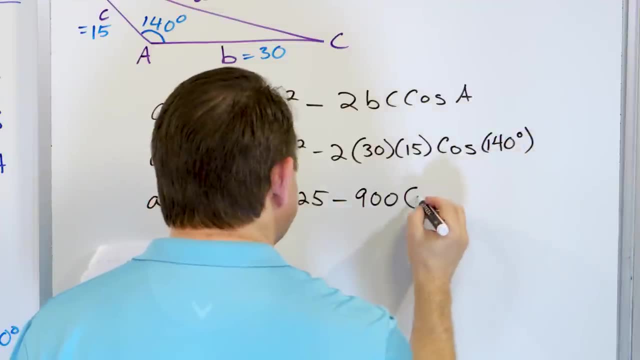 15 squared is 225.. And then the 2 times the 30 times the 15 is 900.. When we take the cosine of 140, we get negative 0.766 in the calculator, And then we have A squared. 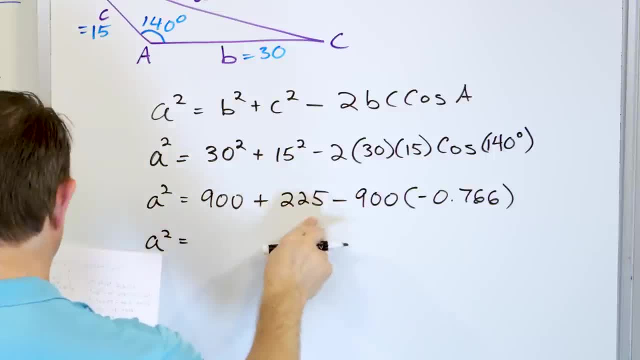 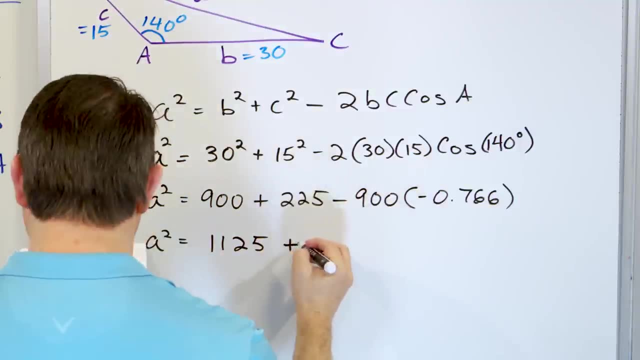 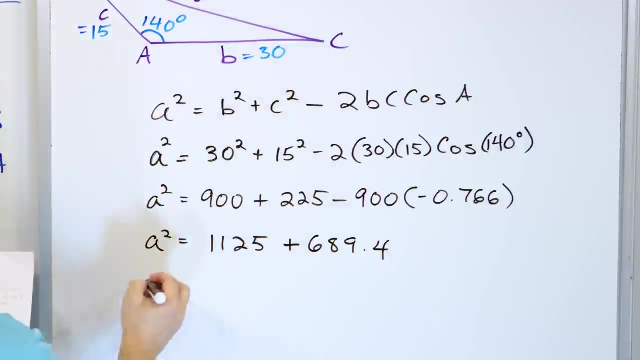 When we have 900 plus 225,, we get 1125.. And then what we have negative times- negative is positive, So this becomes a positive 689.4 when we multiply these together. So we get 1,, 1,, 2,, 5 plus 689.4.. 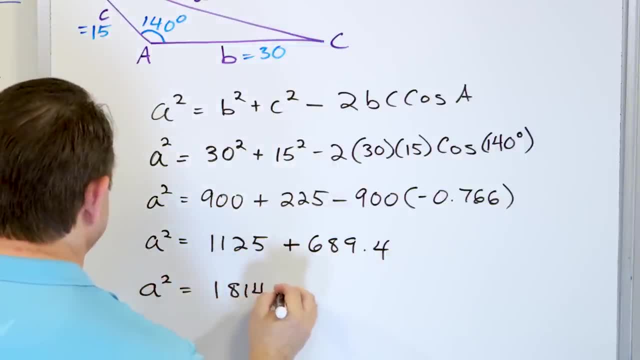 So we have a squared is 18, 14.4.. We add these guys together, but that's a squared. So to get rid of that, we take the square root of both sides. So we take the square root of this. 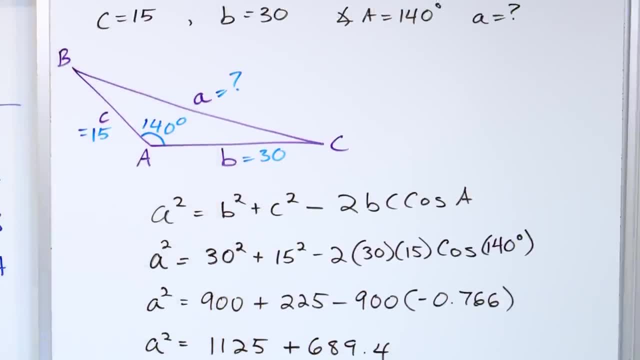 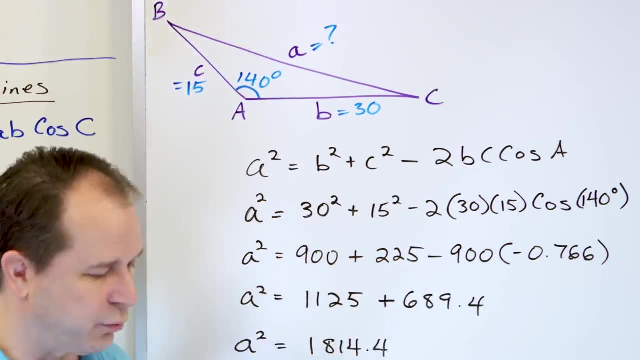 We get 42.6.. That's the answer for the side a, 42.6.. So if this was in centimeters, for instance, then that would be 42.6 centimeters. So now we've introduced the law of cosines. 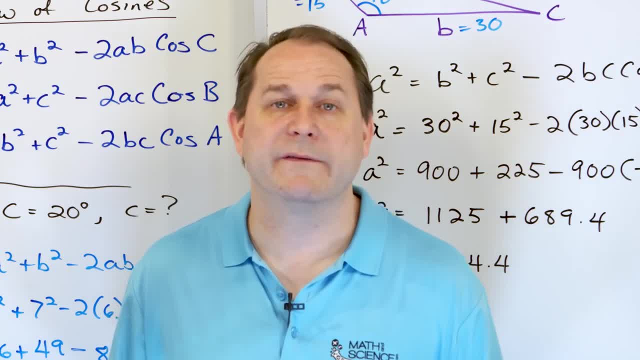 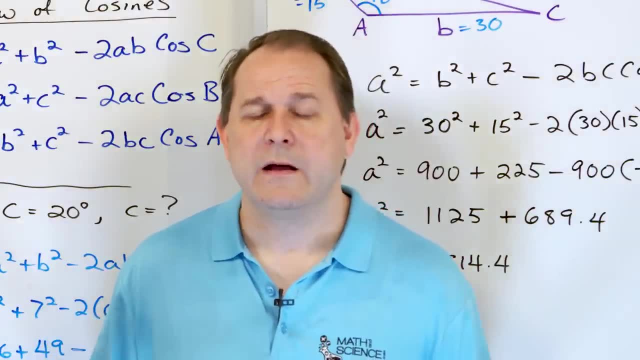 I've tried to encourage you to understand that it's just a modified form of the Pythagorean theorem. that's true for any triangle of any shape with any angles. And then we did two examples to show you how to use it, And normally I don't prove everything, but I want to prove this one for you. 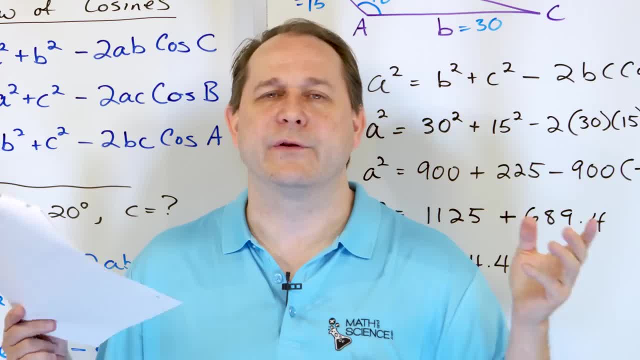 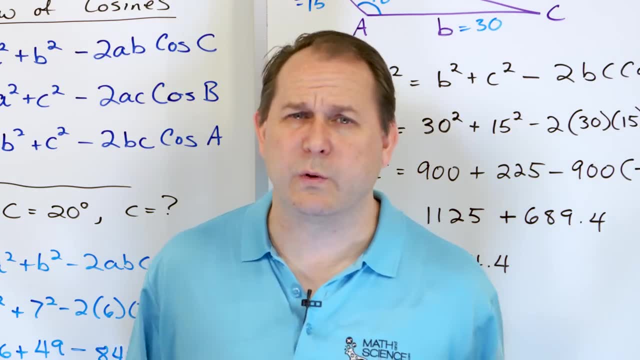 I want you to know where it comes from, but also because the tools that we'll need for the proof, which are not hard, by the way, but they are things that we use constantly throughout math. So I feel like this proof is a really good one, because the things that I'm going to talk 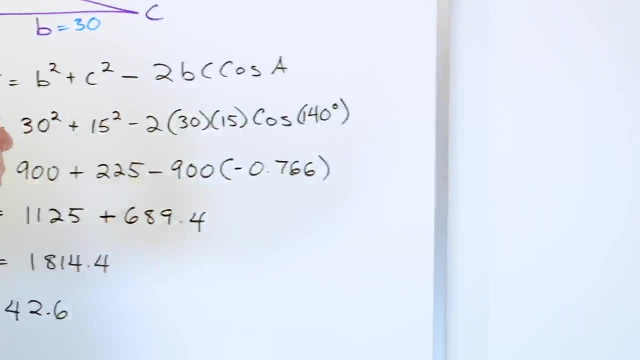 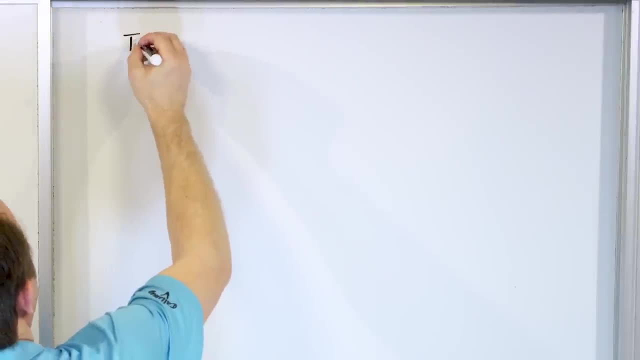 about you're going to use them forever, basically. So let's talk about where this law of cosines comes from. So first I'm going to introduce a couple of tools. Some of you may already know these tools. That's great. 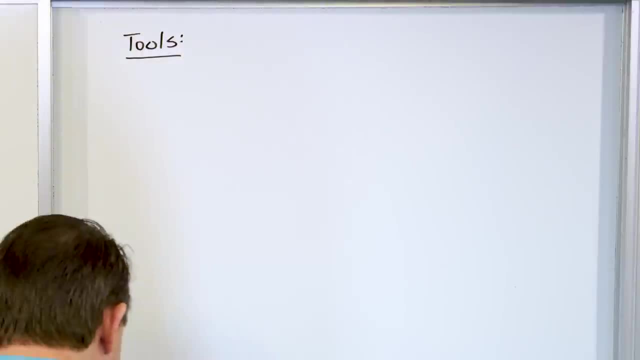 Some of you may have no idea what I'm talking about, but that's okay, because it's very easy to understand these tools anyway. So let's go back to a unit circle, right? What does a unit circle mean? You need this for the proof. 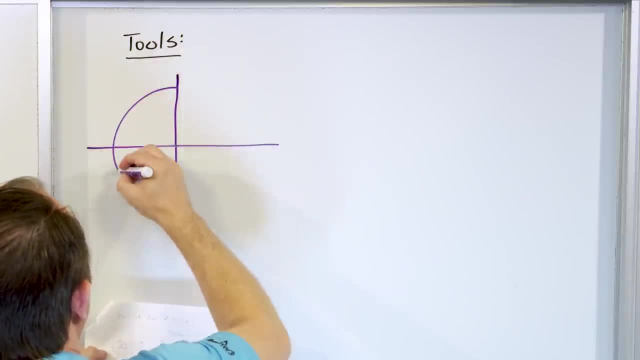 So we're going to talk a little. A unit circle is just a circle centered at the origin that has a radius of one. So that means this is one and this is one and this is negative one and this is negative one. 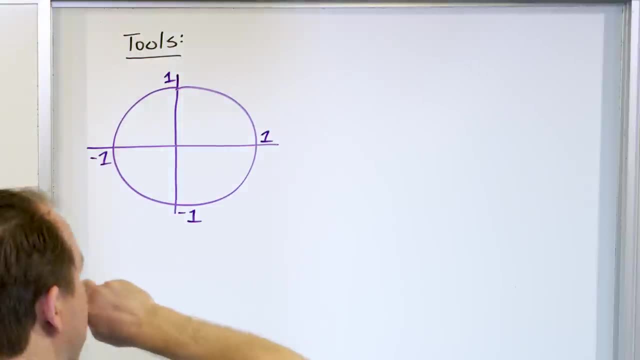 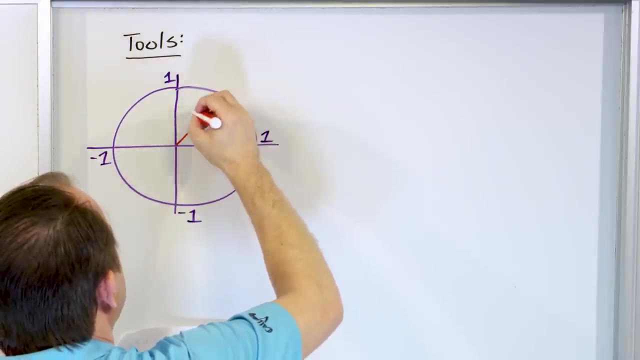 That's what a unit circle is. right Now, we already know all about unit circles from understanding sine and cosine. So let's draw a radius of one because, notice, it's a circle of radius one. So any distance from the origin to the circle has a distance of one, and we can break this. 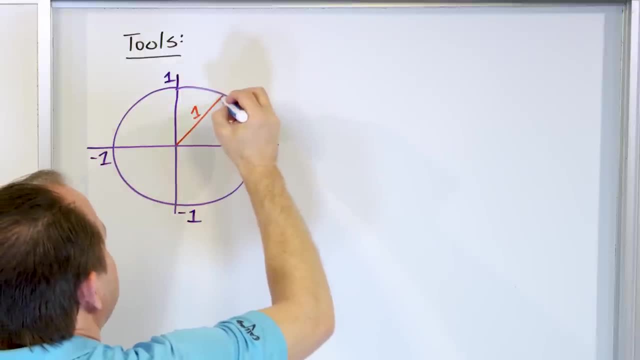 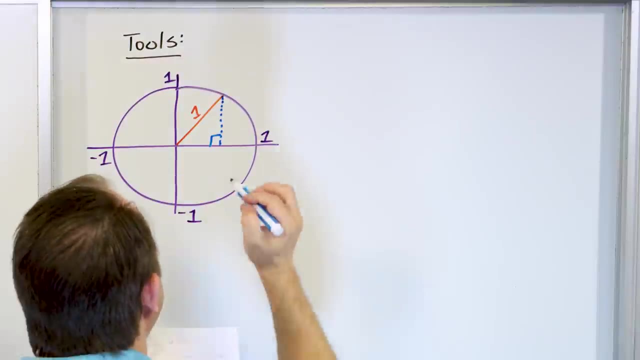 kind of like this hypotenuse or this length. we can split it up vertically into kind of like a make a little right triangle here. We've done this right. That's what we talked about sine and cosine. I've been telling you over and over again that the vertical side here is, if this is, 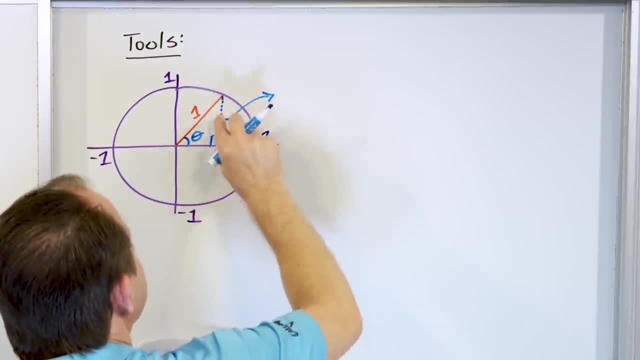 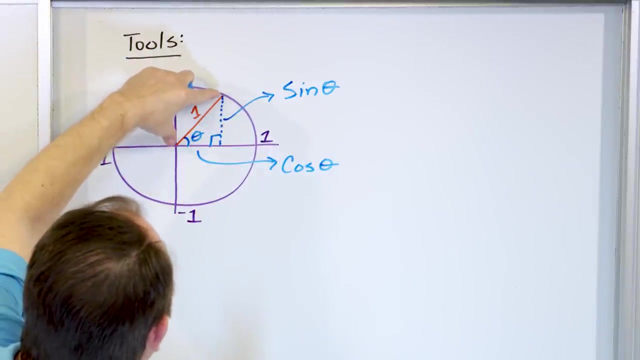 an angle of theta right where it's up there like this that this vertical side of this triangle here is called the sine of the angle theta and this distance right here this is called the cosine of angle theta. So basically, if you have a unit circle with a hypotenuse of length one and you know the, 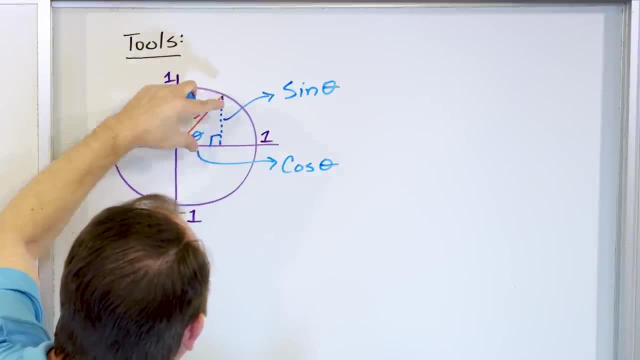 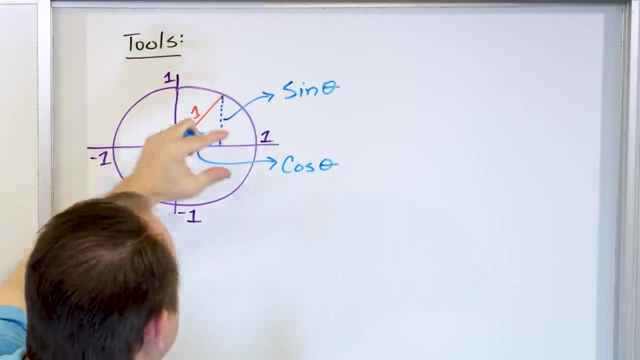 angle here. if you take the sine of the angle, you get the length of this triangle which is just literally the hypotenuse of one. it's shadow projection onto the y-axis, basically right here. How much of that hypotenuse, kind of fractionally, is existing in the vertical direction. 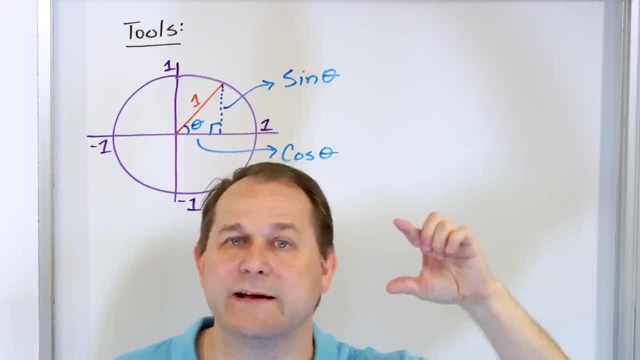 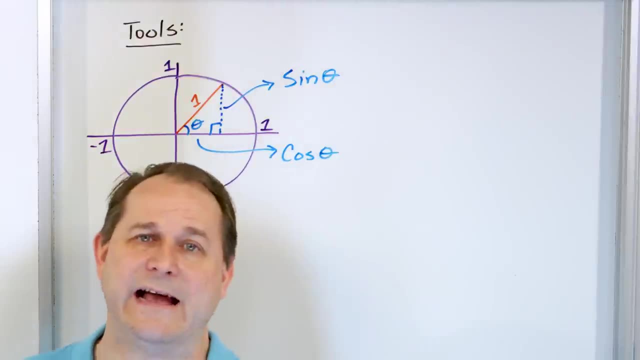 That's what you're doing. You're taking the shadow projection along the y-axis right. That's what the sine of an angle is. The cosine of an angle is sine of an angle. It's taking the shadow projection of that hypotenuse onto the x-axis. 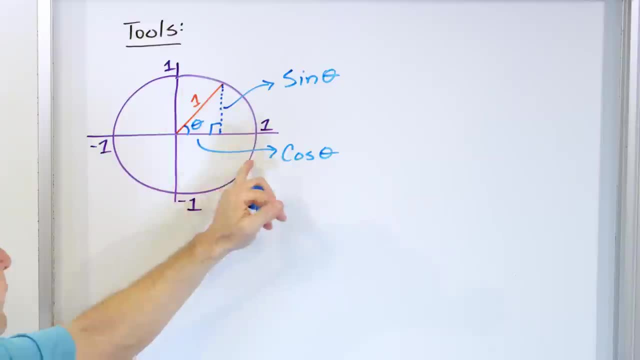 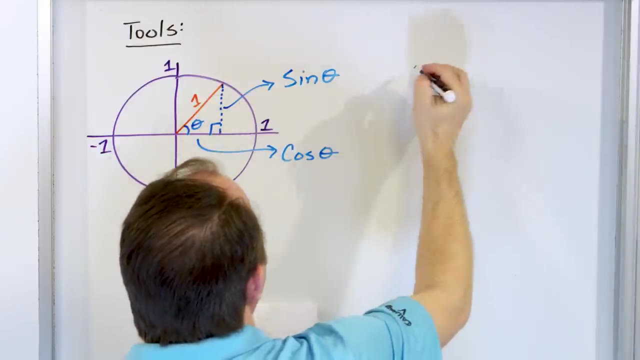 So that's why we call it the x component and the y component when the hypotenuse is one. But we know that this is a right triangle in here, and so we know that the Pythagorean theorem holds for any right triangle. So we know c squared is always equal to a squared plus b squared, because this forms: 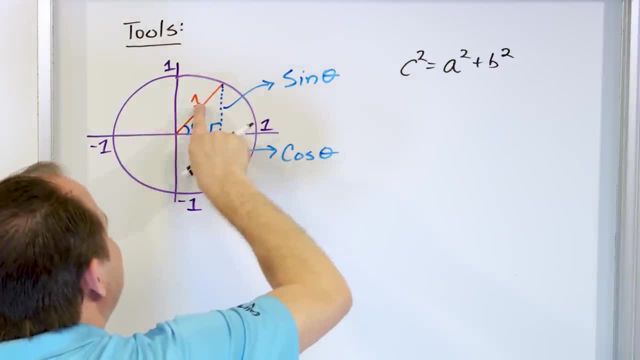 a right triangle. But what is c in this case? It's just the length of one. It's a unit circle, So we can put the length of c being one squared. And what is side a? Well, side a and b can be either one of these guys. 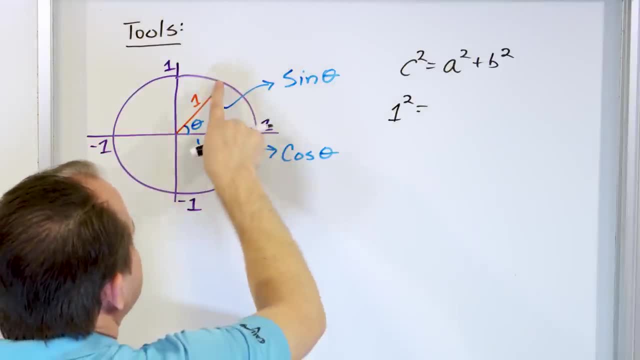 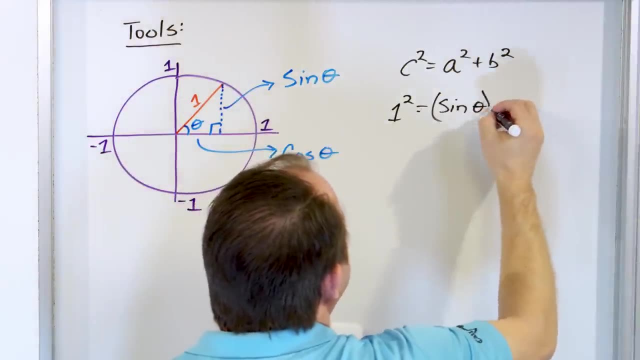 But you can see that side a. you can consider let's call it sine here sine, So sine of the angle. We just said this side of the triangle was sine of the angle. We can put it in for the value of a. 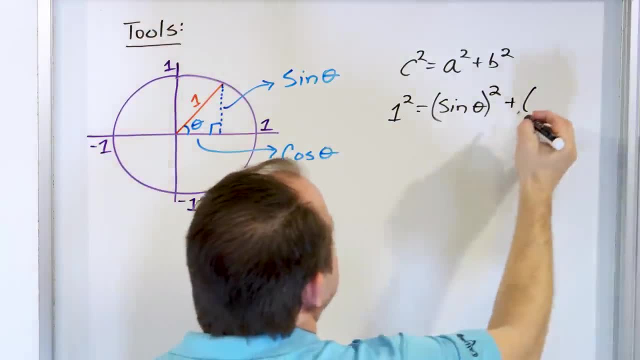 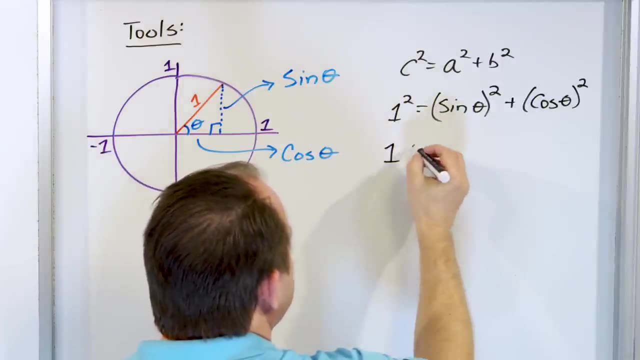 And then the value of b, the other side of the triangle. we already said it's the cosine of the angle. So it's the cosine of the angle and that's squared. So what have we figured out here? That we have one, squared is one. 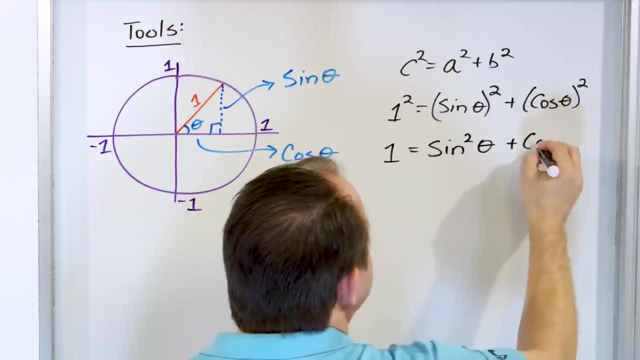 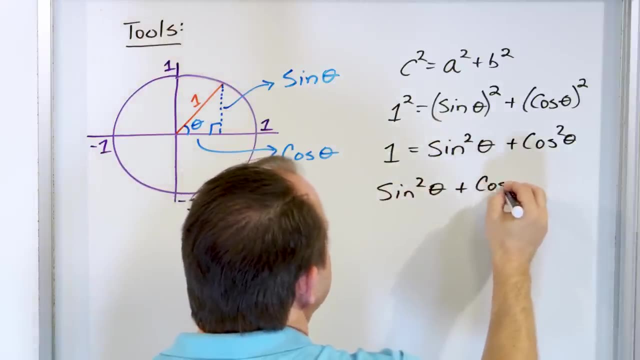 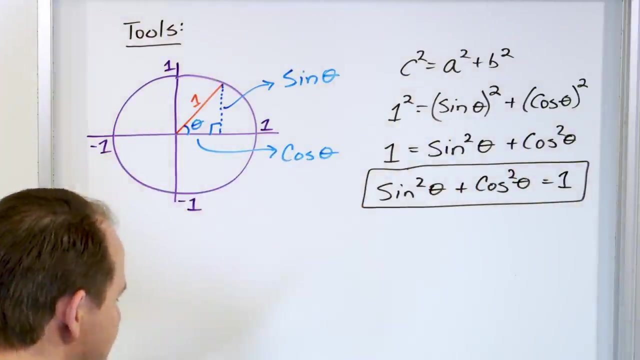 And this we can write as sine squared of the angle, And this we can write as cosine squared of the angle. Let me flip it around: Sine squared of any angle plus cosine squared of any angle is equal to one. This is an identity that we're actually going to learn a little bit later in class. 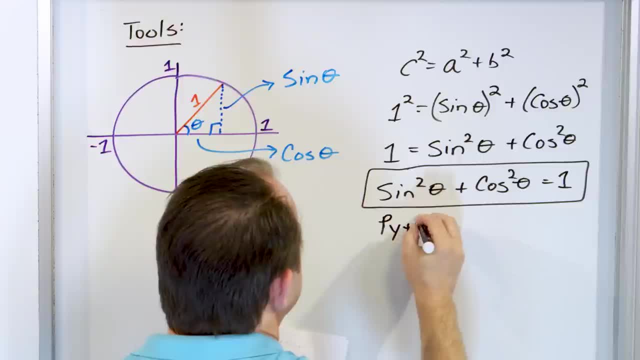 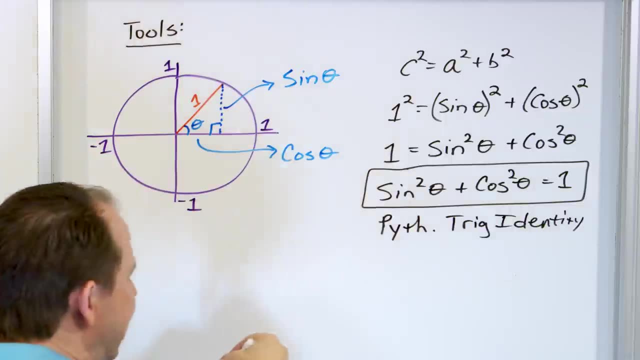 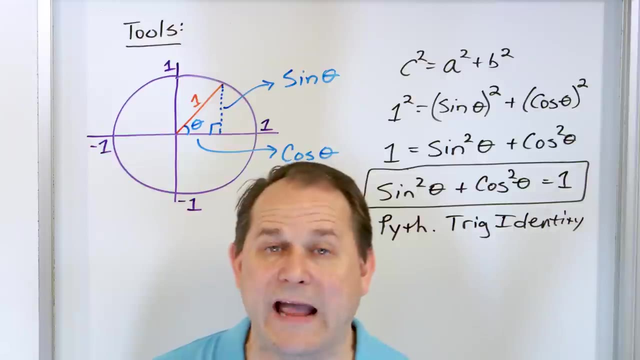 It's called the Pythagorean trig identity. Pythagorean trig identity. Do you know why it's called the Pythagorean identity? Well, it comes straight from the Pythagorean theorem. Anytime you have a unit circle, you always have a 90 degree angle in there. so you have 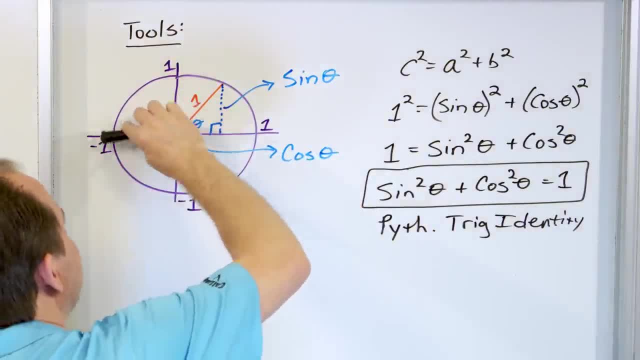 a right triangle, So for any angle around the unit circle, no matter where this thing points. if you take the y projection here, which is the sine of the angle, and the x projection, which is the cosine of the angle, no matter what the angle is, they're always going to add up. when 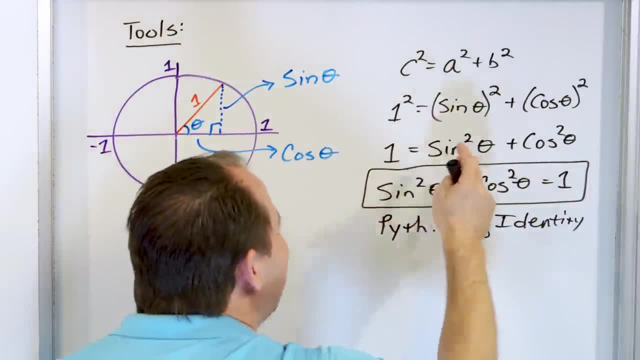 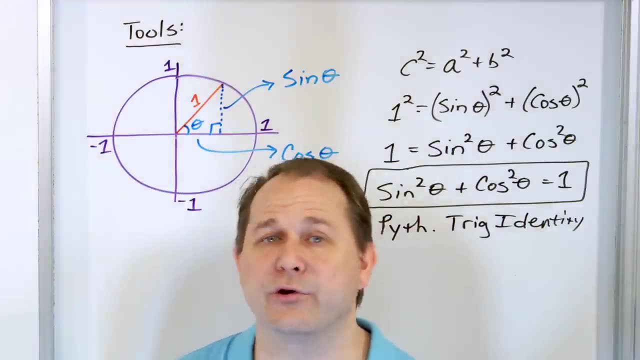 you square them to the number one. So sine squared of any angle plus cosine squared of any angle always equals one. Always Grab a calculator, Pick any angle you want- 87.2 degrees. Take the cosine 87.2 degrees. 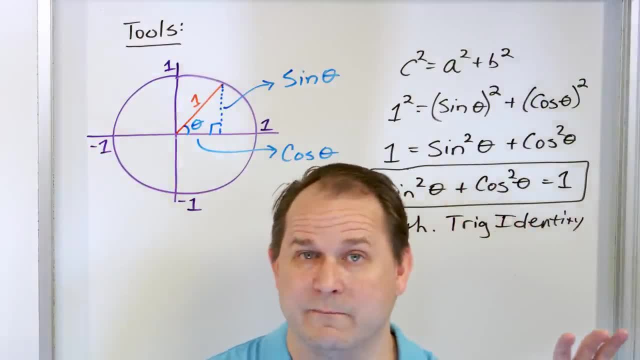 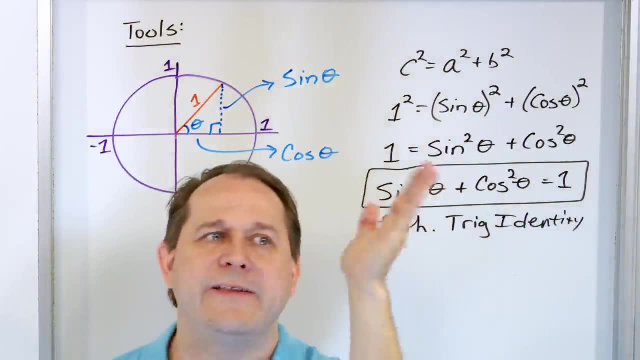 Take the sine, Take both of those answers and square them and add them together And you're always going to get one for any angle. because the unit circle. and what sine and cosine are? they always form right triangle And because of Pythagorean theorem, they always when you square, you know when you take the. 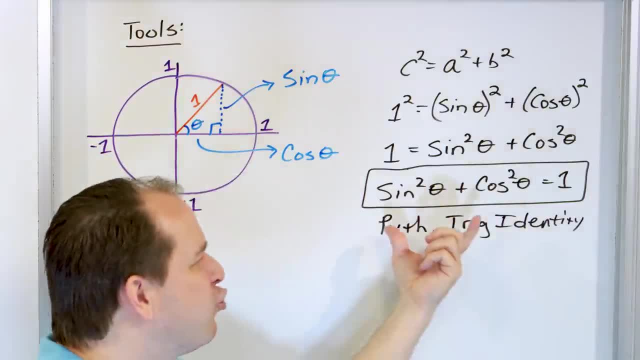 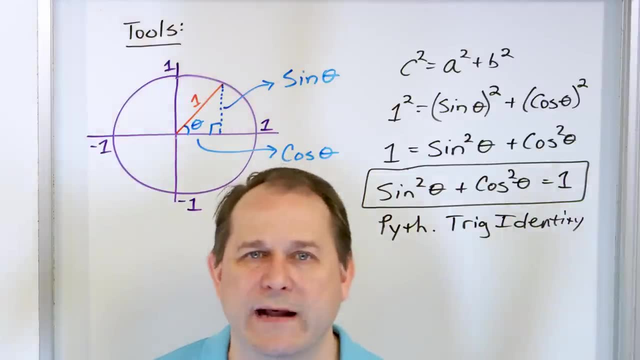 values and you square them, they're going to always add up to one. So this is incredibly useful. In fact, if I had to pick, like, one trig identity, if I just had to pick one and say that's the one I really, really, really want you to remember, this might be the one because 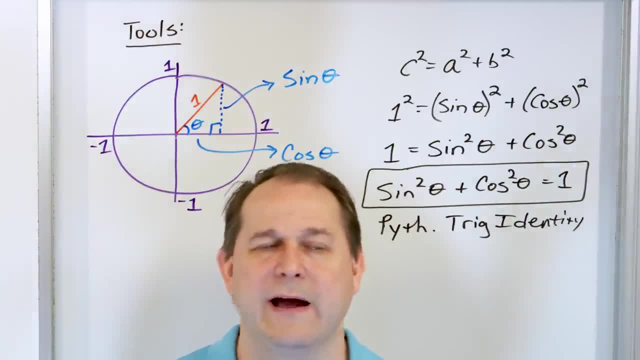 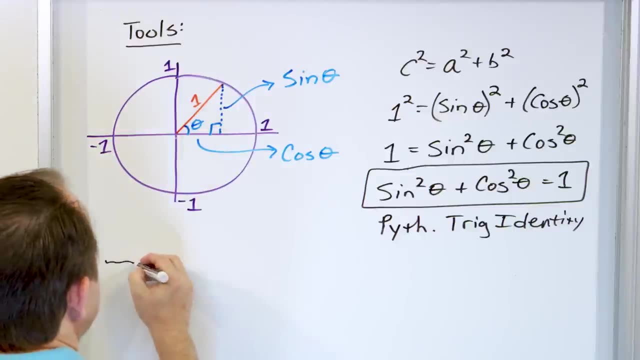 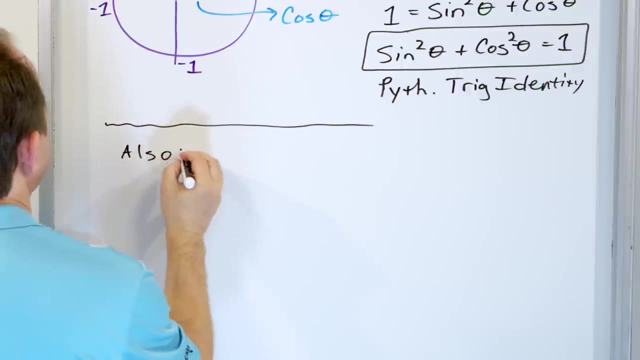 it's comes up everywhere in math. It's always true, And it's so fundamental because it comes from Pythagorean theorem. Okay, So that's tool number one. Let's talk about tool number two Now. the second tool we're going to need- I'll put also- is basically pretty much as important. 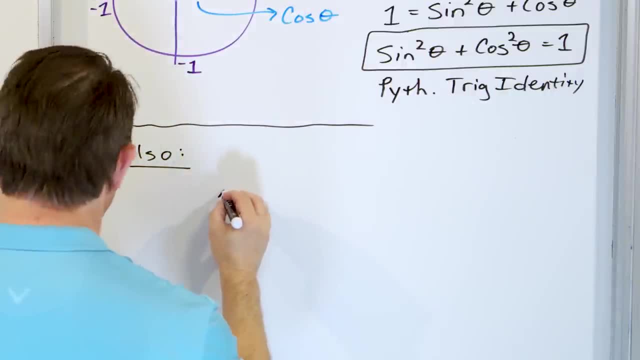 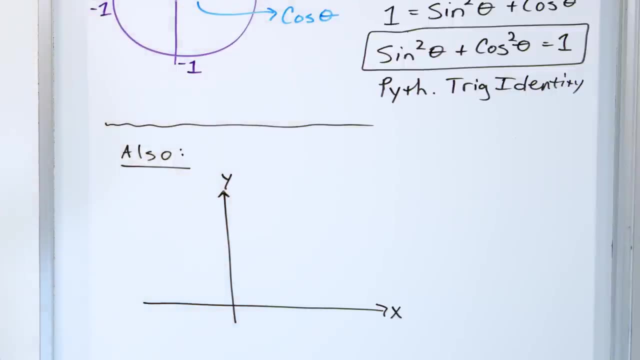 as this. We use it a lot in more advanced math classes. It's very simple to understand, So let's draw A little X- Y axis right here, and we'll need both of these to understand where the proof comes from. Let me pick a point anywhere in this X- Y plane. 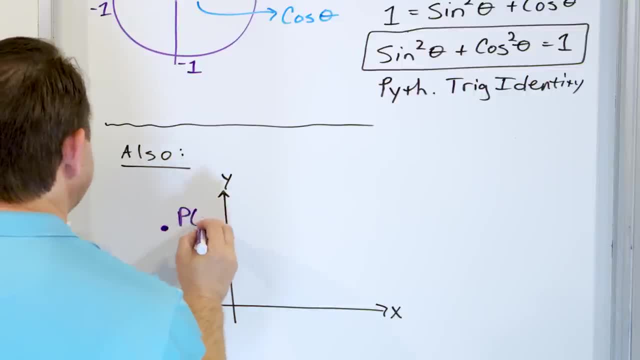 Let me pick it over here And I'm going to say that this is some point and it has coordinates X comma Y. That's why I have parentheses X- Y. The point P has coordinates X comma Y. Now what I'm going to do is draw an arrow which goes from the origin through this point. 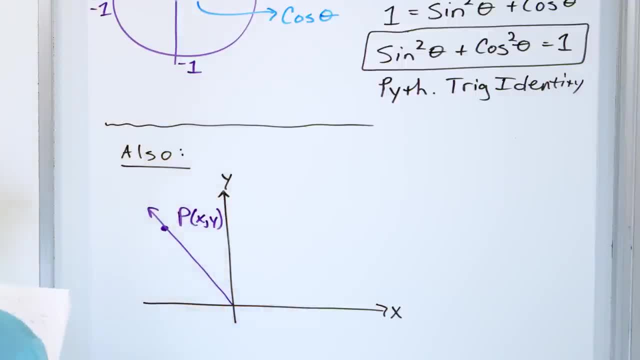 like this. It's supposed to be a straight line, but it might be a little bit curved. Okay, Now this. This line is what forms the, the angle where this point exists, the angle to the X axis, right here. Okay. 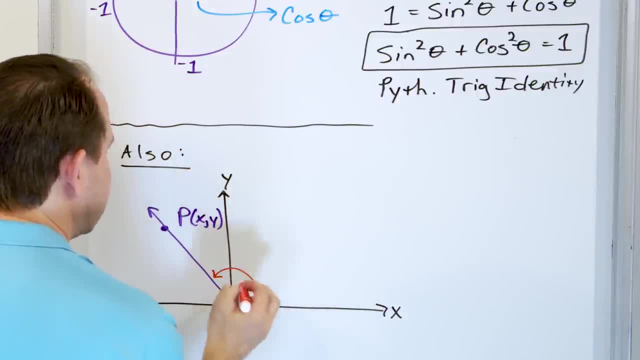 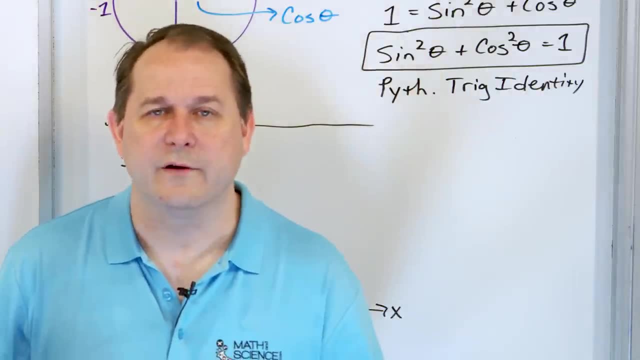 And so there's an angle from the X axis to this little line here, and we're going to call this angle theta. So what we're dipping our toes into we're going to get into a little later. It's called polar coordinates. 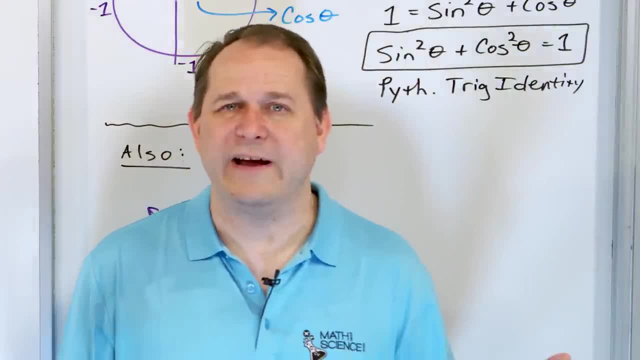 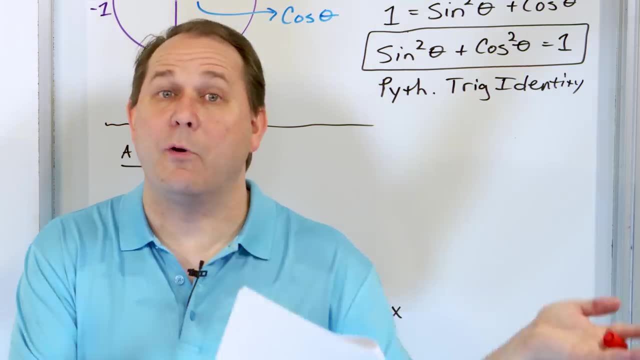 Okay, And I'm introducing it now because we have enough information to understand it and we're going to use it in just a second, but it's very simple to understand. when you have a point on the plane, you can represent it as X, comma, Y. 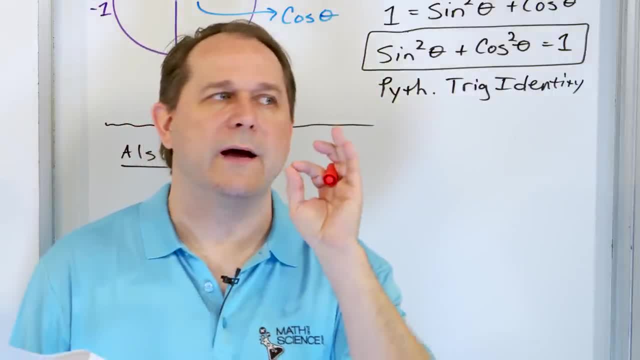 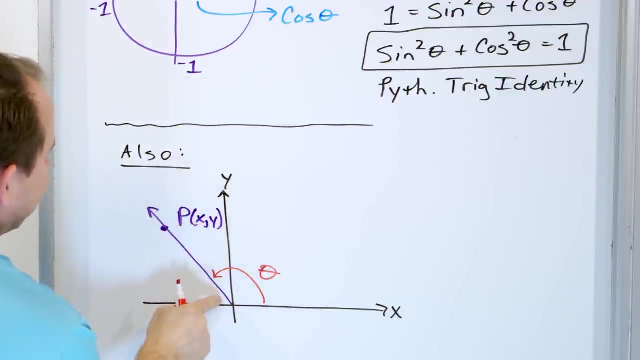 That's great. It's X- Y coordinates, but you can also specify its location by drawing a line from the origin through it and telling me where the angle is. so you can, I can tell you how far along this line it is in this direction. 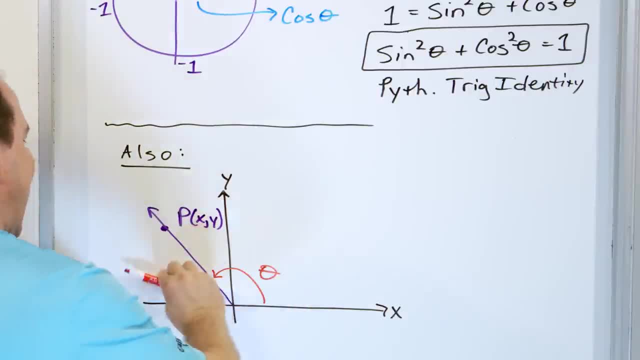 And then also the angle and any point in the plane. I can tell you the angle of it and its distance from the origin, And I can also specify its location anywhere there. Okay, But notice that this point also forms a right triangle. Big surprise. 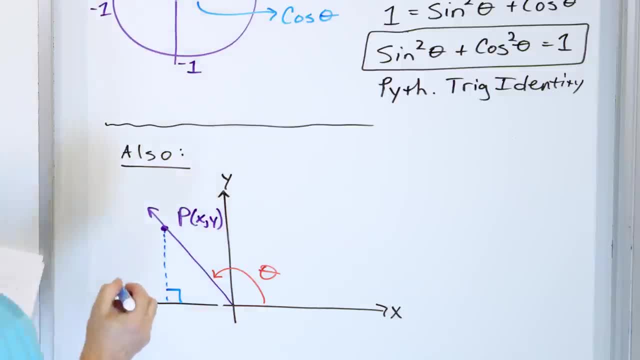 Right, We're going to do that all the time, right, And we already know that. if I tell you, the distance from this point to the origin is R. like I already told you a second ago, we can specify the point two ways: X, comma, Y or. 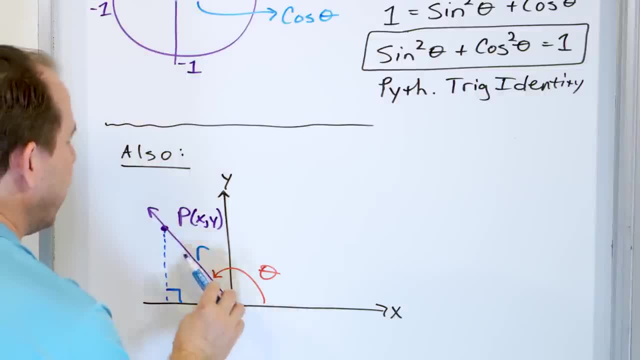 a distance R from the origin, however many centimeters from the origin and the angle from the X axis, If the point's here it might be R could be two centimeters and the angle might be 140 degrees. If R is maybe over here, you know, then maybe, or if the point is over here, maybe the distance 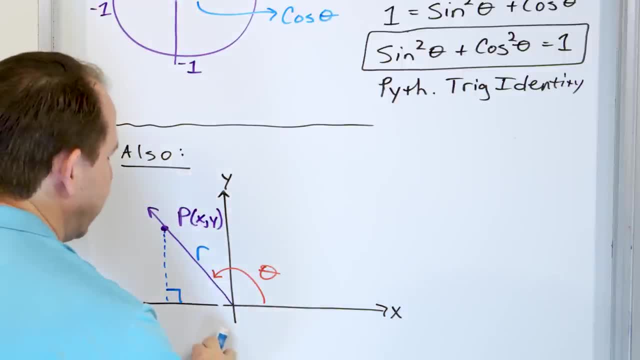 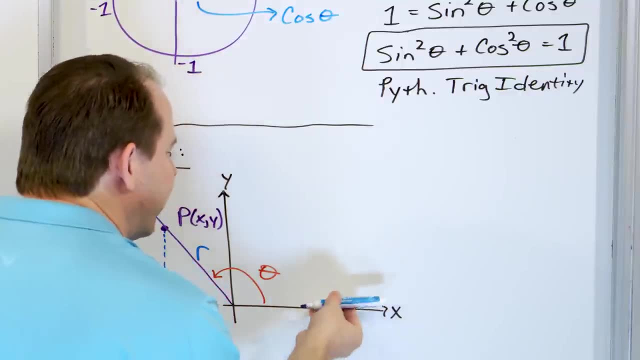 from the origin is three centimeters and the angle is like 230 degrees. If the point's like way over here, then maybe the the R. the distance from the origin is like 10 centimeters And it's at an angle of all the way around to 350 degrees, almost 360 degrees. 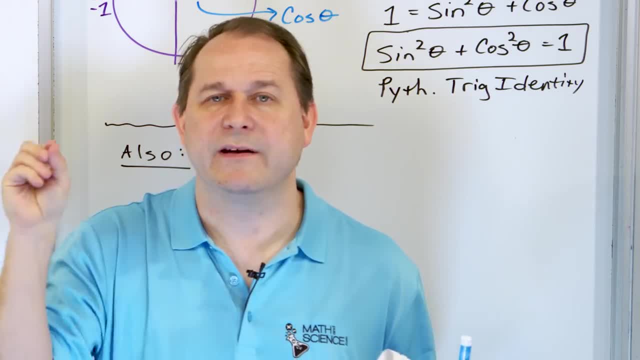 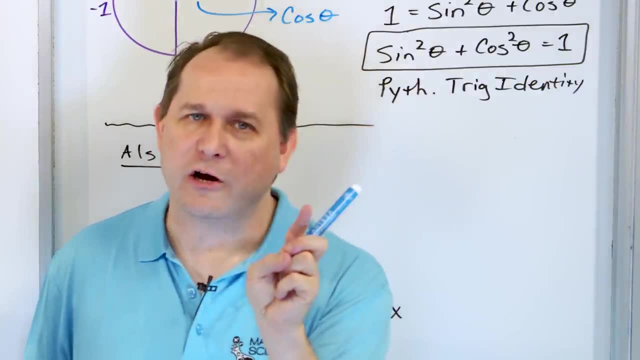 So you always need two points or two numbers to represent a point in an X- Y plane. You could just give me X comma Y, or you also could give me two different numbers, R and theta. Theta tells you the angle where it's at. 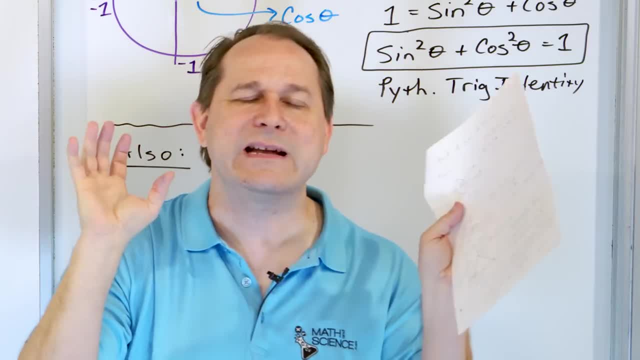 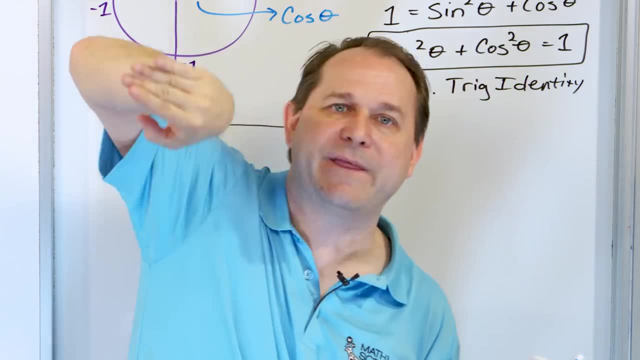 And R tells you how far away from the origin it is And you can uniquely identify any point anywhere in the X Y plane with those two numbers are the distance from the origin and some angle theta from the X axis. All right, So that's why I put R here. 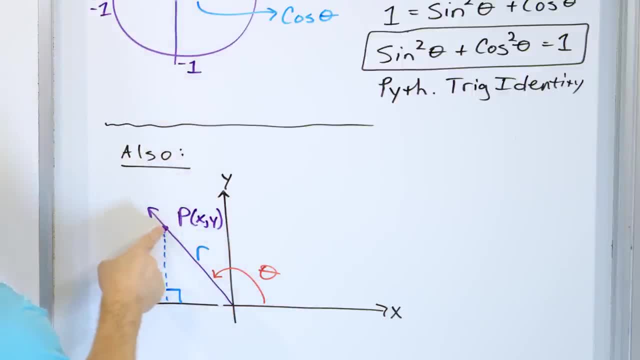 It's the distance away from the origin, And at some angle here that also could be the definition of where the point P is. But we know right. we know that if this is true, then this side of this triangle is R. 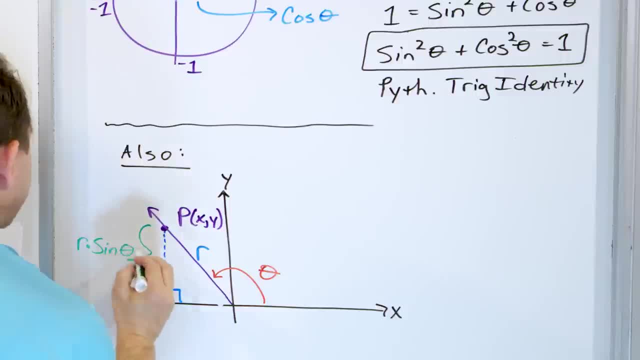 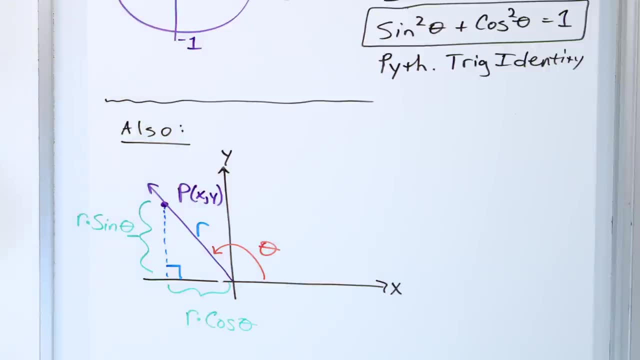 We know that this is R multiplied by the sine of theta And we know that this distance here is R multiplied by the cosine of theta. How do we know this? Because the cosine of the angle theta here, or the cosine of the angle theta, is the adjacent. 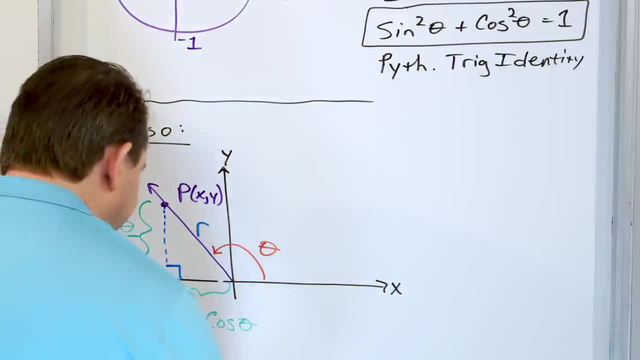 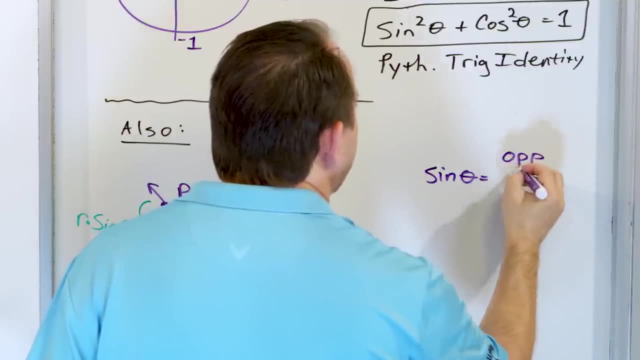 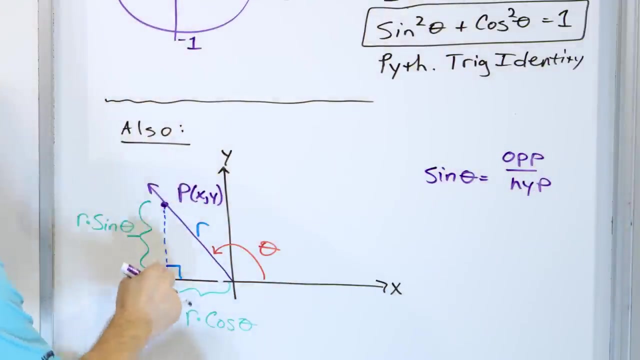 side over the hypotenuse And the sine of the angle. I guess I can go over here. You can say that the sine of an angle is its opposite over the hypotenuse. But the hypotenuse is R right, So the opposite side, which is this side of the triangle, can be written as the hypotenuse. 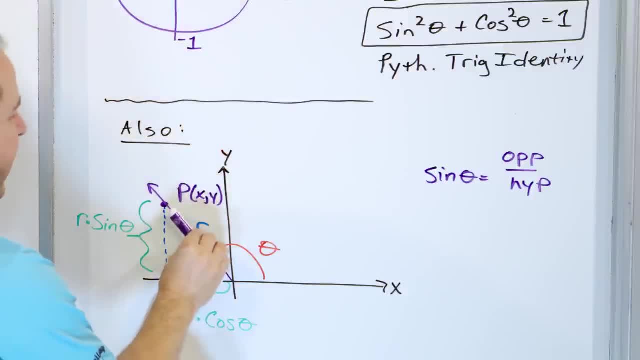 times the sine of theta. Basically, what we do is we say: however far this distance is to give me this side of the triangle, I just take it and I multiply by the sine of the angle which chops it into the Y direction. 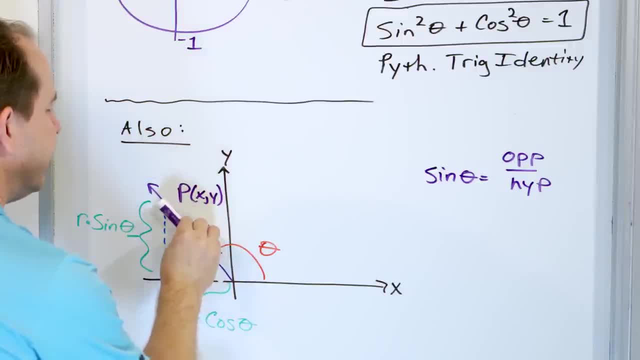 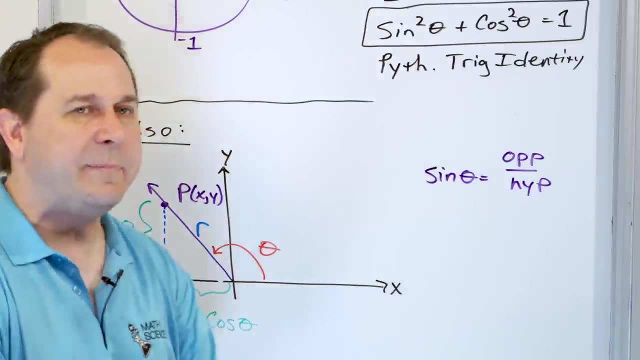 To find this distance on the X axis, I take this distance of the number and I multiply by the cosine, So R times the cosine chops it into the X direction. I've been telling you that cosine and sine are like chopping functions the whole time. 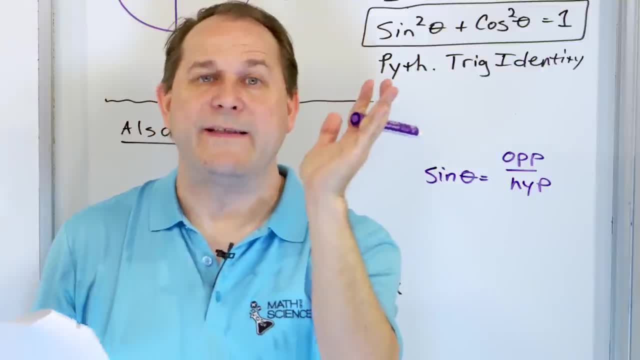 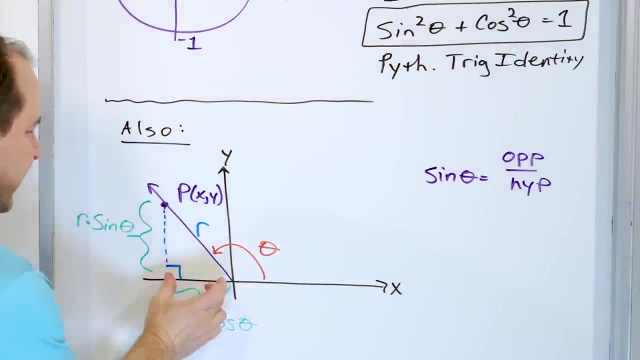 So if you know a distance from the origin and you multiply by the cosine of the angle where it is, then it chops it and tells you the horizontal distance on the X axis. like this, It chops it and tells you the shadow projection down here. 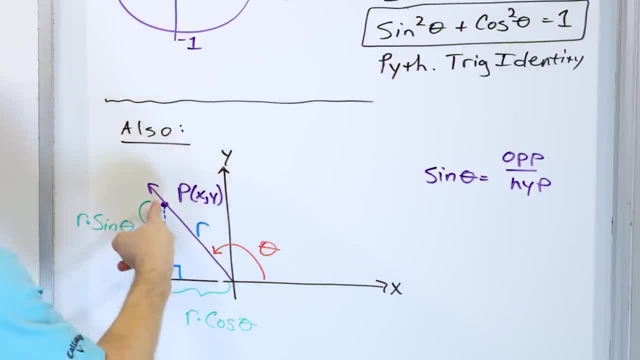 If you take the distance R times the sine of the angle, it gives you the shadow projection into this direction. This is what we've been doing all the time. So once we know that we've got this Okay, That we can do this, then we can specify the point two ways. 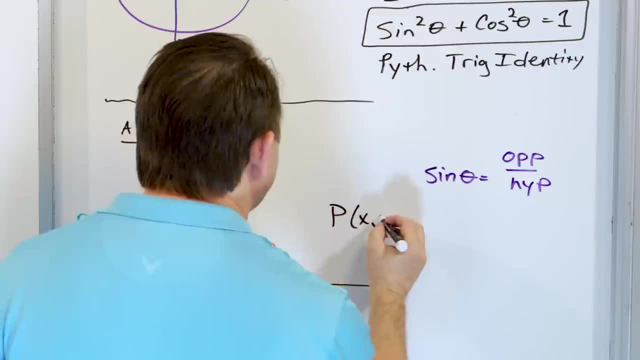 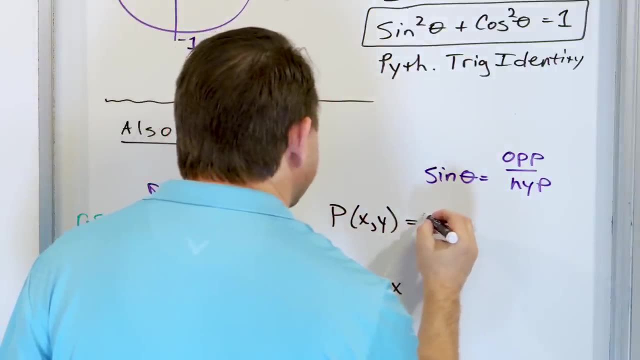 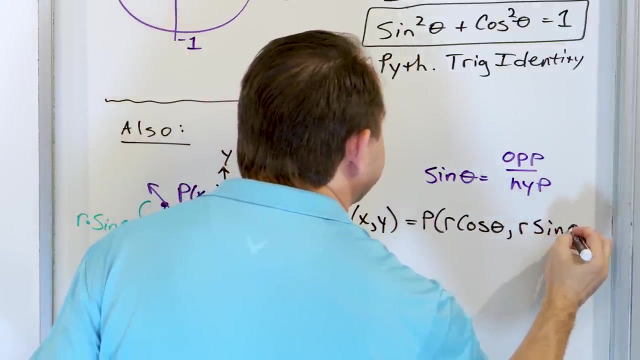 P can be specified in an X comma, Y fashion. but if the X coordinate of this point P, we can write it as R times cosine of theta and the Y coordinate can be written as R times the sine of theta. What we're basically saying is this point: it forms a triangle, right? 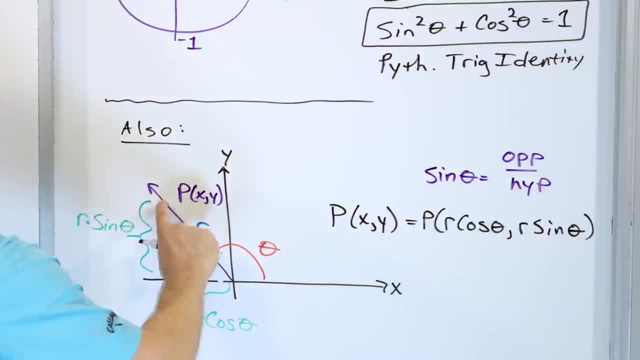 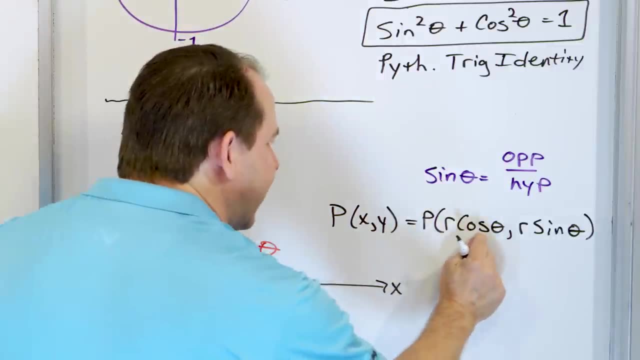 And we just said that this side of it was R times, the cosine of theta, and this side was R times, the sine of theta. So the X coordinate, which is this, literally this coordinate along this axis, is R times cosine of theta. So the X component can be written as R times, the cosine of theta, and the Y component of 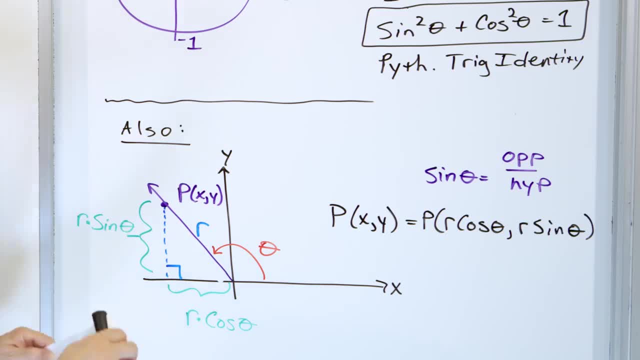 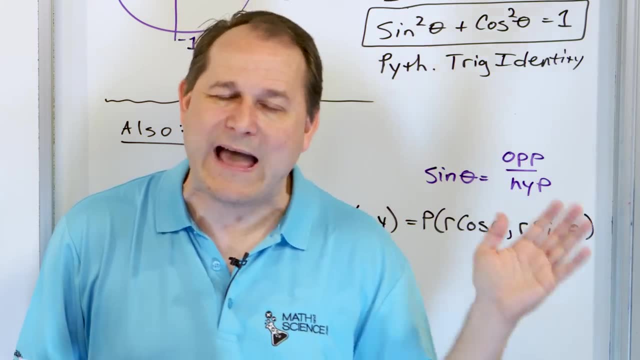 this point can be written as: R times the sine of theta. So I'm getting a little bit into polar coordinates because we're going to be doing a lot more with it very, very soon. but we have enough now to write down our proof of the law of. 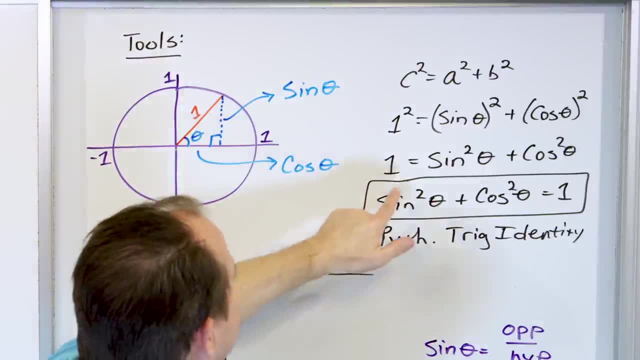 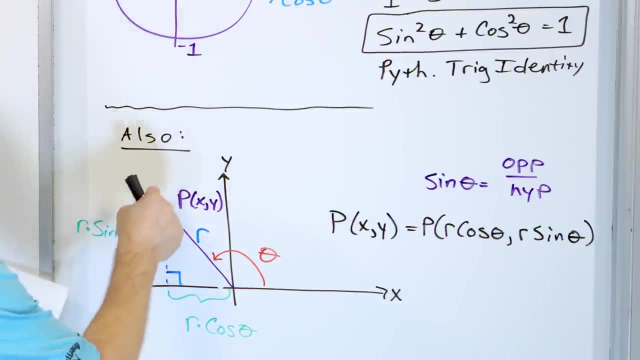 cosines. All right, So two things. First time you have an angle sine squared plus cosine squared is one. That's fact number one. Fact number two: any point in the X- Y plane can be written as an X- Y coordinate pair. 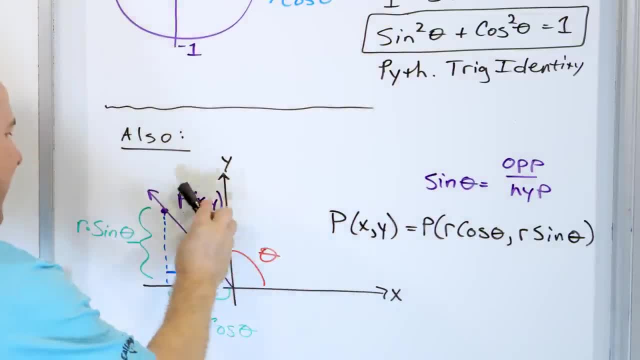 but the X coordinate can be written as R times the cosine of the angle it makes with the X axis, And the Y coordinate can be written as R times the sine, because R times the cosine gives you the X projection and R times the sine gives you the Y projection. 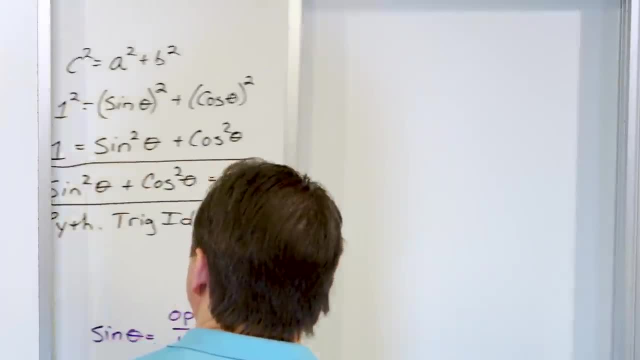 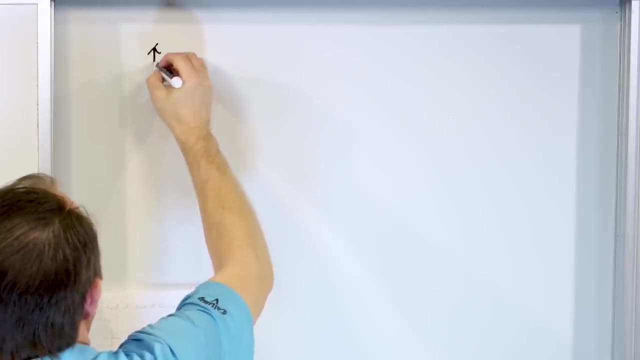 And those are the X- Y coordinates that we have. So now let's do the proof of the law of cosines. So I build it up so much. It seems like it's so difficult, but really it's really not. So let's go ahead and do that right here, and we're going to draw this like this: 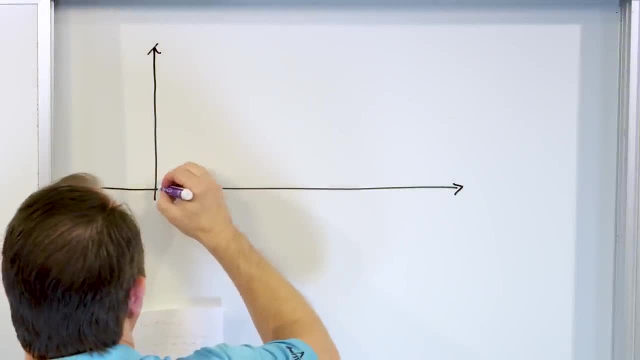 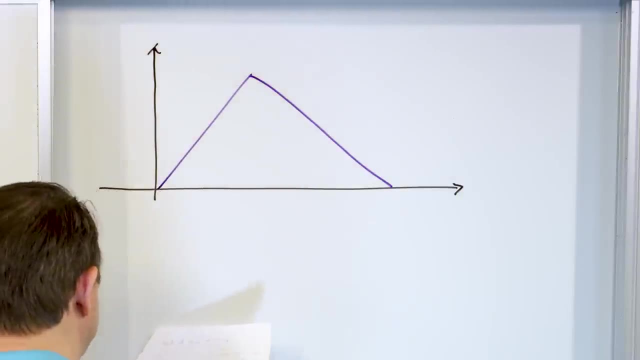 Now what we're going to do is we're going to draw a general triangle. A general triangle goes up and then maybe goes down, like this: There's no 90-degree angle. I'm not giving you any 90-degree angle there. Okay, 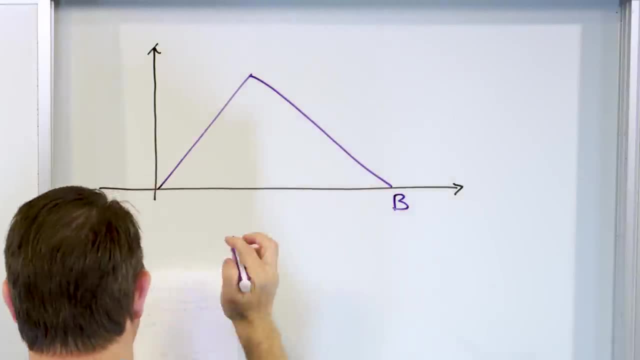 So we can say that this is point B or angle B. We could say this is angle C and I'm going to call this point P. I guess you could call it angle A, but I'm going to call this point Okay, Okay. 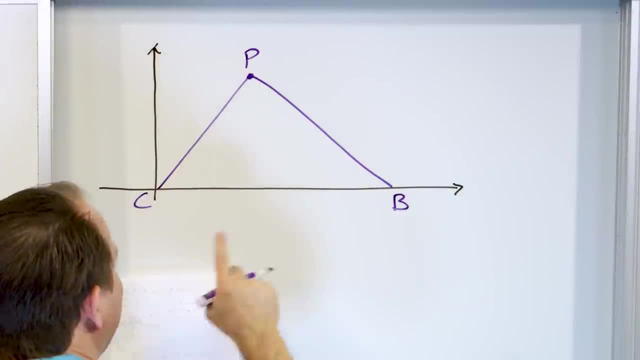 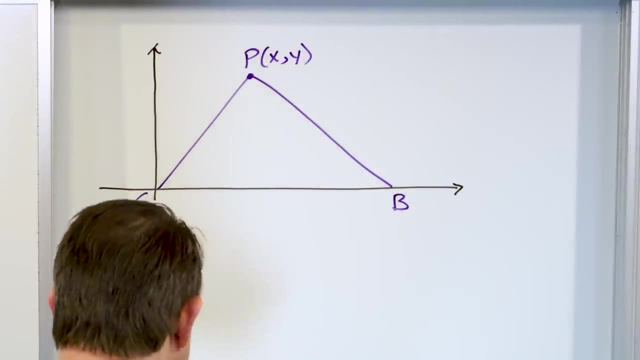 Okay, point P here, or I guess you could just say that this is point C and point B and this is point P here, and it's x comma y right, x comma y. Now we also know that this angle is angle C, right here. 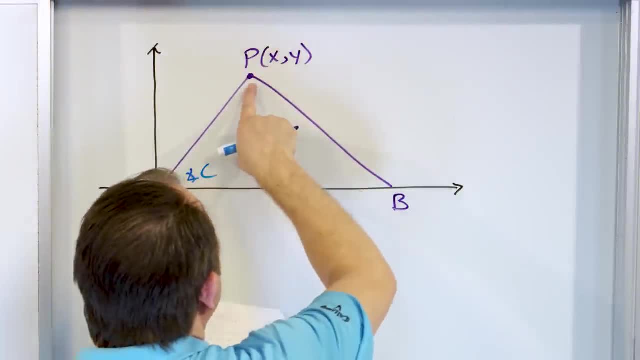 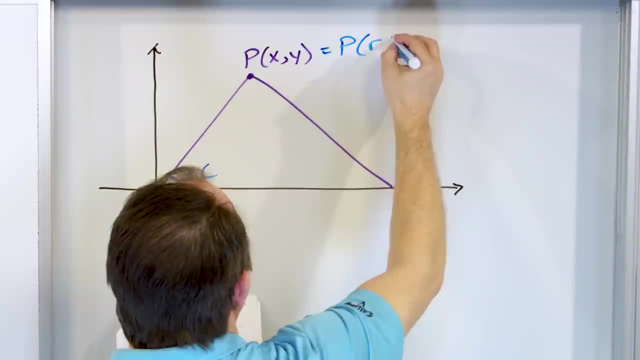 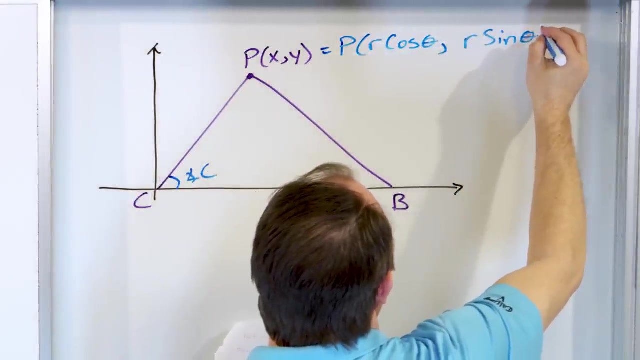 all right. So this xy point, any point in the xy plane, any point, the x coordinate can be written as r times the cosine of whatever the angle is, and y can be written as r times the sine of whatever the angle is. Now you might be telling me, like well, what are you talking about? I'm 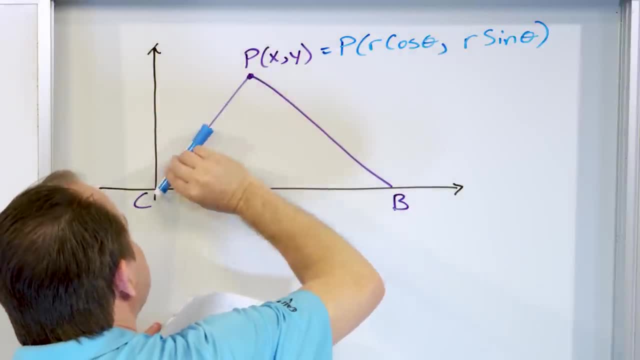 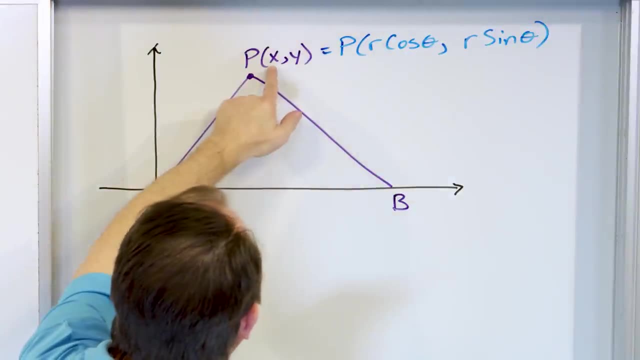 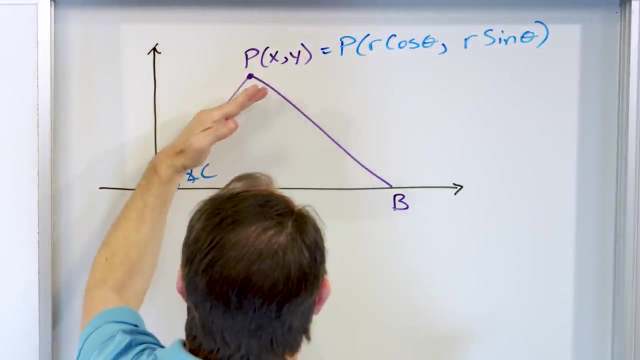 saying that this point P you can write it as a distance from the origin at some angle and this angle is going to end up being angle C right here. but in general you can say that the x coordinate is going to be can be written as the distance r times the cosine here and then the y coordinate. 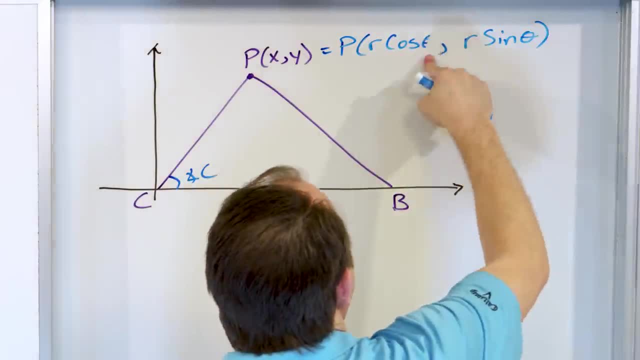 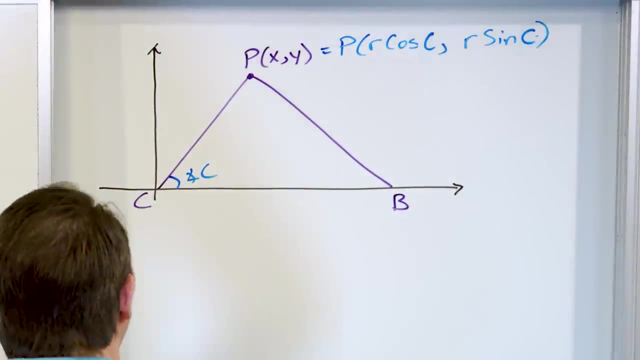 is r times the cosine. So this is the x coordinate and this is the x coordinate and this is the r times the sine. all right, So actually, instead of putting theta here, I'm going to erase theta and I'm going to say that this is actually angle C. So let's talk about why, because 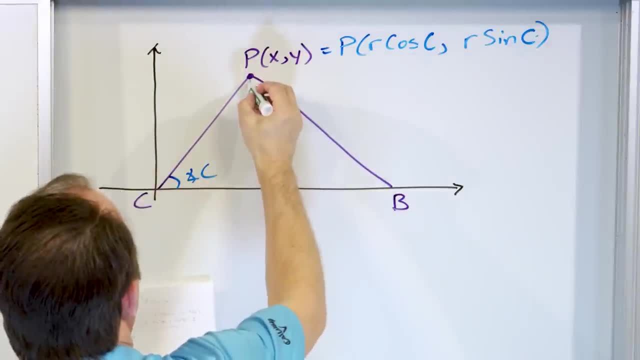 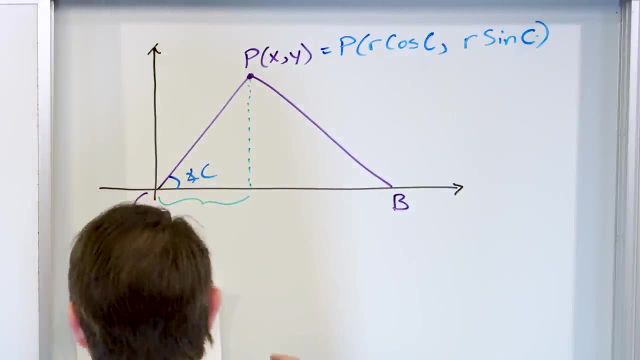 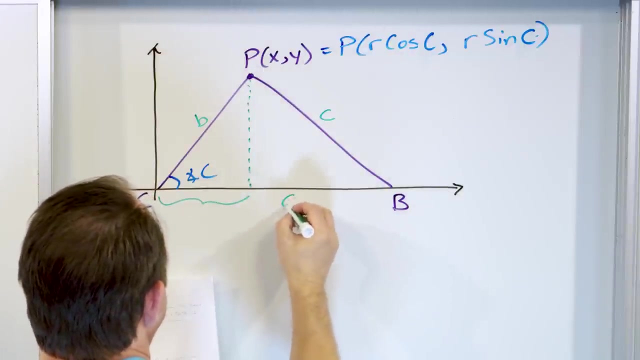 if I draw a little dotted line down here, I'm saying that this distance right here is, this distance right here is, if this is side B and this is side C and this down here, this whole entire distance here is. I'll just put A right here. 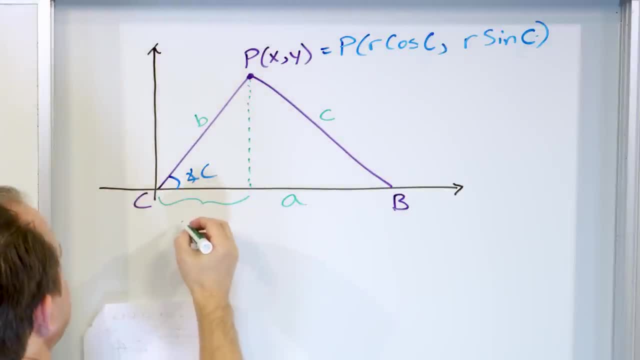 the whole distance here, then this distance right here is B times the cosine of angle C, B times the cosine of angle C, And this distance right here when I go over here, this is B times the sine of angle C. So make sure you understand that. All I'm saying is I'm 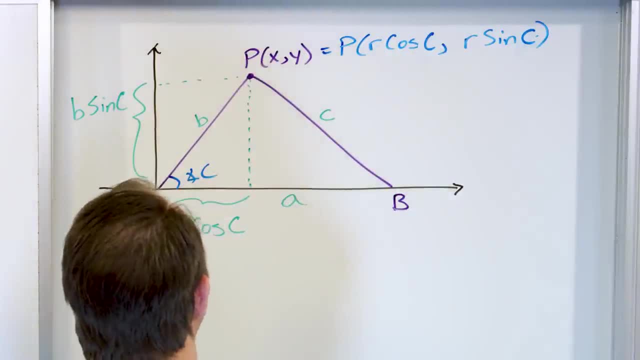 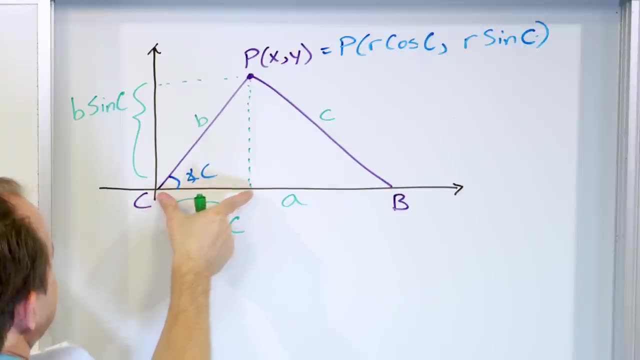 drawing a triangle here. here's a point, and this is what we're going to use to prove the thing. but if you know that the length of this side of the triangle is B, then B times the cosine of this angle is going to give you this distance, and B times the sine of this angle is going to 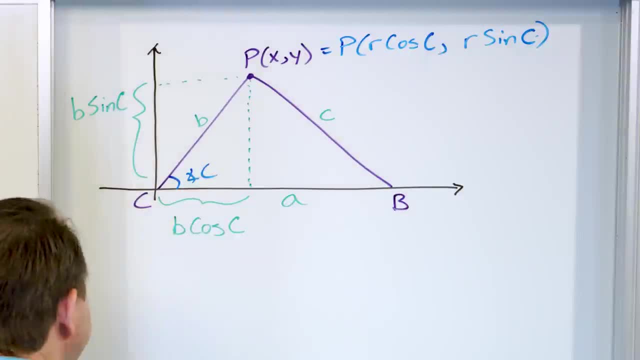 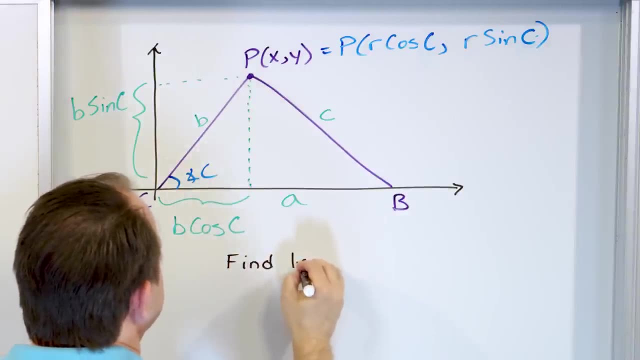 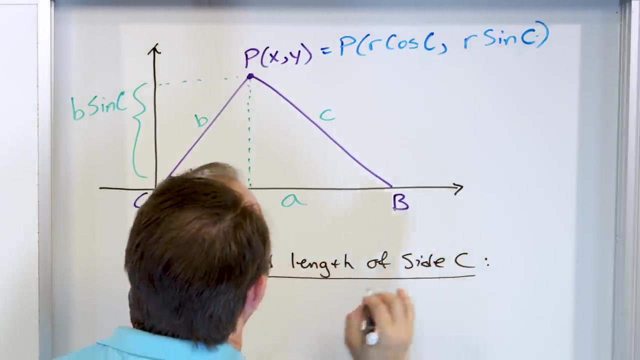 give you this distance. Now what we want to do is use the Pythagorean theorem. I want you to tell me the length of C, So find. this is going to prove it for us: find length of side C. Find the length of side C. So we're going to use the Pythagorean theorem. So we're going to say: 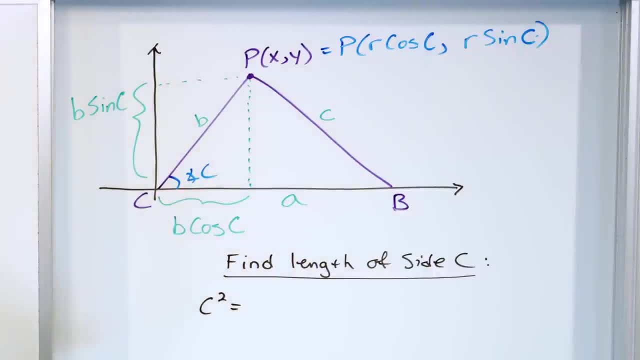 that C squared is equal to A squared plus B squared, right. But if this is C, then what is the other side of the triangle? We have this side right here and we have this side right here, All right. So if we want this side of the triangle, 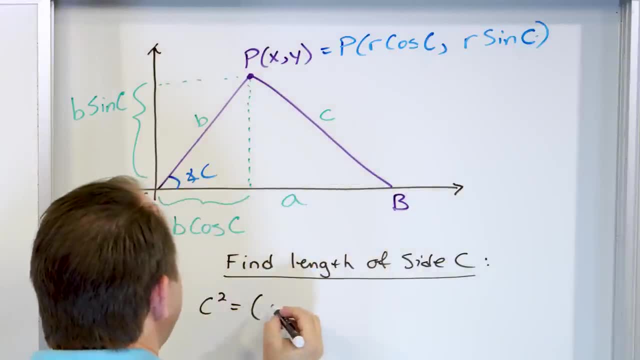 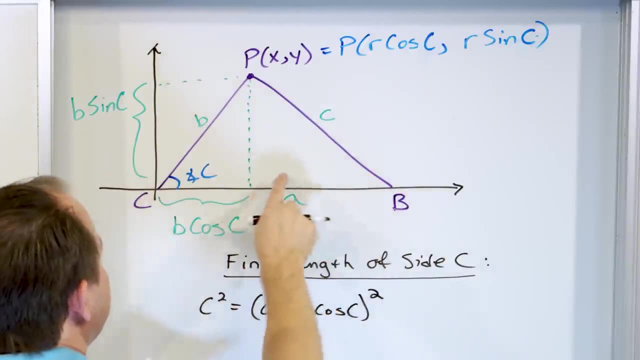 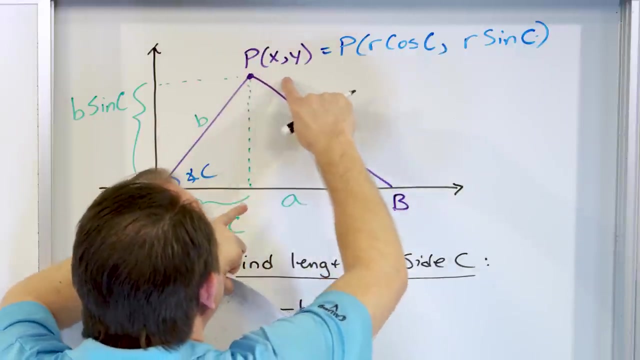 if A is the entire length here, then what we have here is A minus B, cosine of angle C squared. That would be just this side of the triangle. The entire side is A minus. this little side gives us this. What we're trying to do is find the length of this side. So C squared is this. 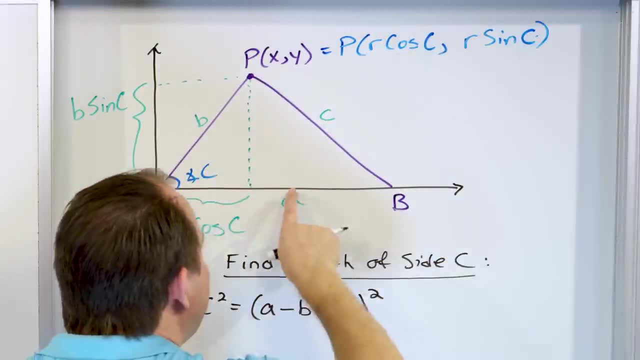 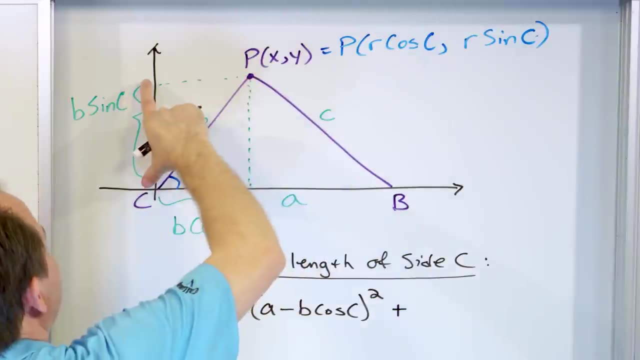 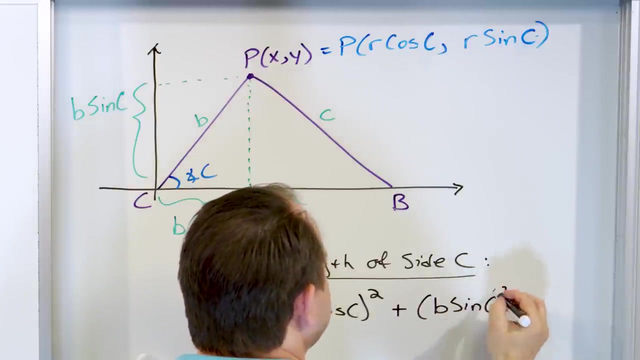 side squared plus this side squared, But this side is the entire length A minus B cosine C squared right. And then we have the other side of the triangle, which is given right here B times the sine of C squared. Make sure you understand this before we go on any farther. 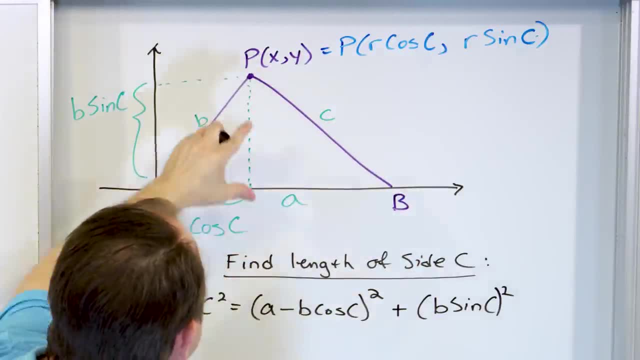 I'm just saying that we're going to find the length of side C. It's going to be the other side of the triangle, this squared, and it's going to be this side of the triangle squared, But this side of the triangle squared is the 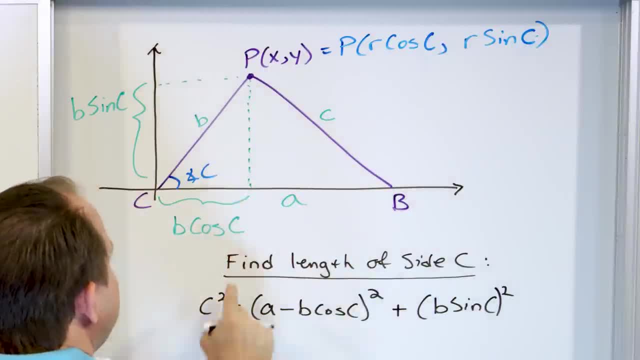 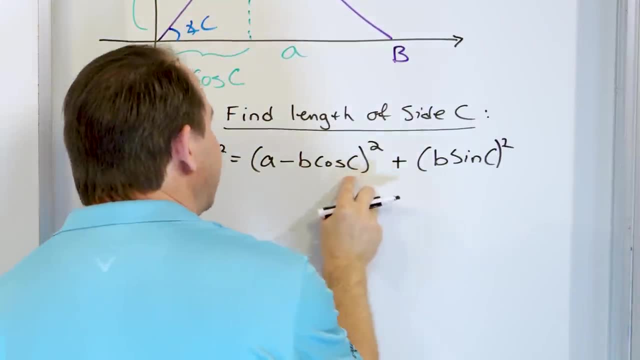 whole length A. A is the whole length minus this little bit, And so that is what is squared. This is really all we need Now. we have to just do the math. So C squared is equal to. now we have this binomial. we got to square it. It's the first term. squared A squared. 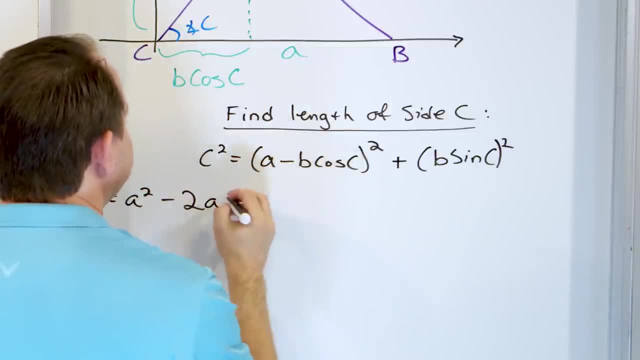 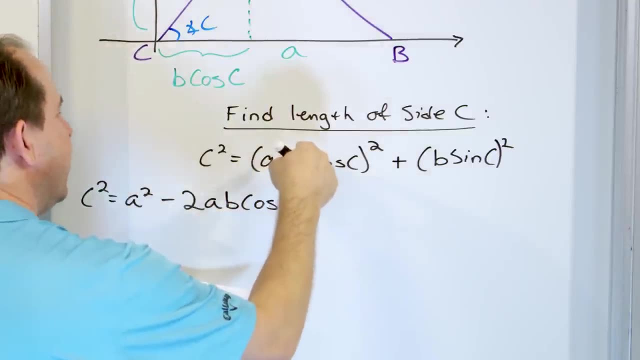 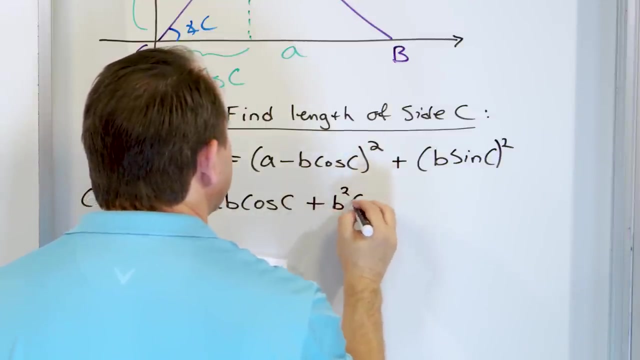 minus two times A times B. So A then times this stuff B cosine C, right. So A squared minus two times A times B, right. And then we have to go plus this stuff squared. when we square it we get B squared, cosine squared C, right, B squared, cosine squared C. 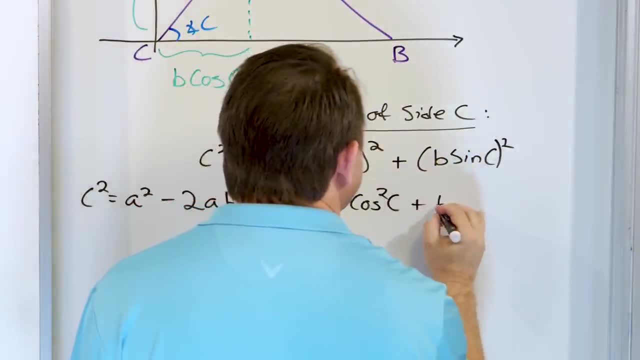 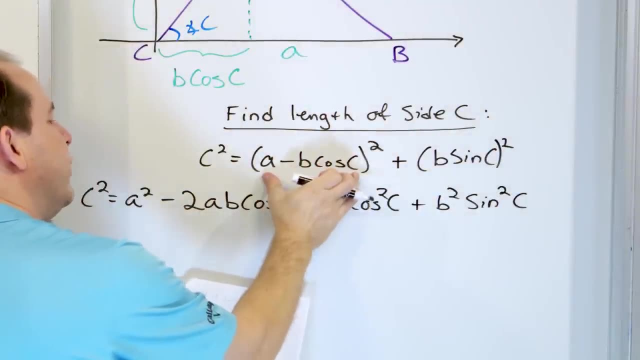 And then finally, we have this one. We're going to square every term inside of here: B, squared sine, squared C. So we remember: square every little term inside. So for this we had to do a binomial, you know we have to do FOIL, basically. So it's the first term squared. 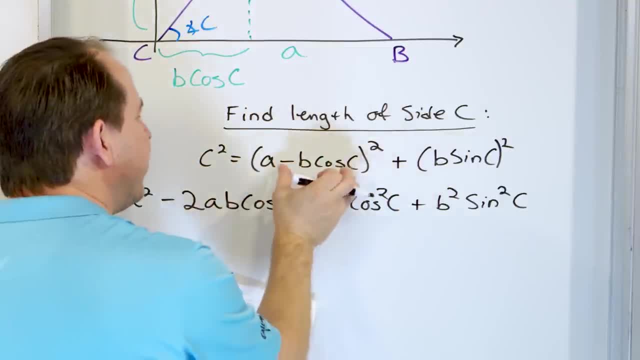 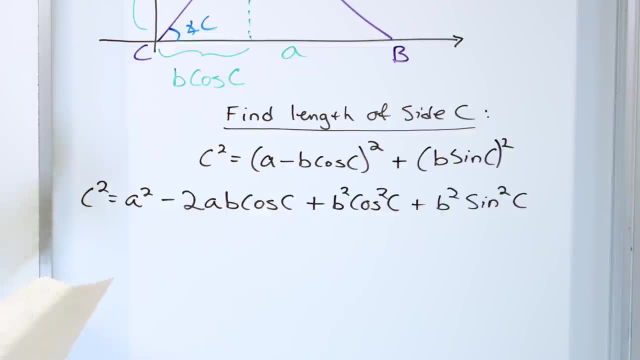 minus two times the first term, times the second term. Then we squared the second thing, So it becomes plus this squared. Then we have this squared. All right, we're getting there. I know it seems very, very much like we're not, but we're getting there. Now we want to group terms together: C squared is going. 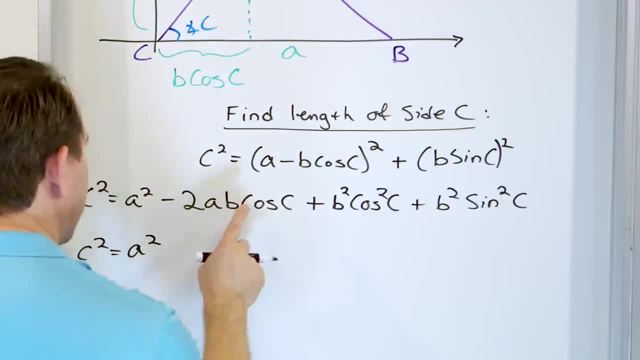 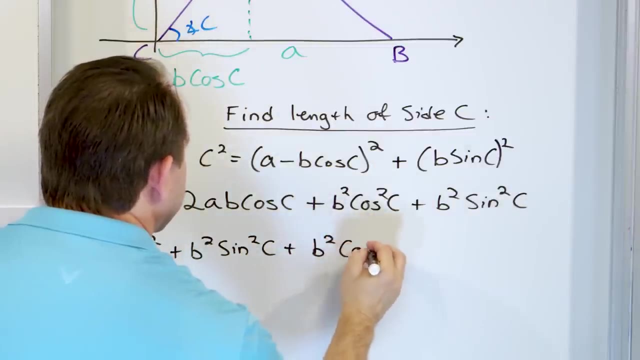 to equal A squared, all right. And what I'm going to do next is I'm going to write this term and this term next to each other. So what I'm going to do is I'm going to write B squared sine squared C- that's this term, plus B squared cosine squared C- that's this term. And then I'm going to write: 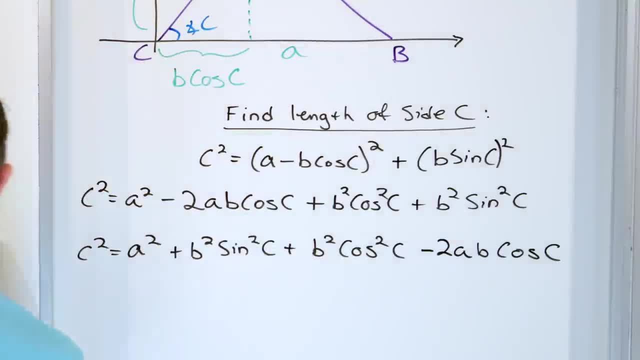 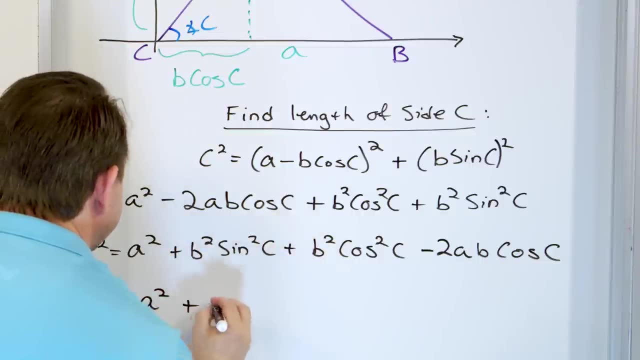 minus two AB cosine of C. all right. So what do we have here? We have A squared. We have a B squared. We can pull it out, We can factor that out. So B squared on the inside. what do we get? All that's. 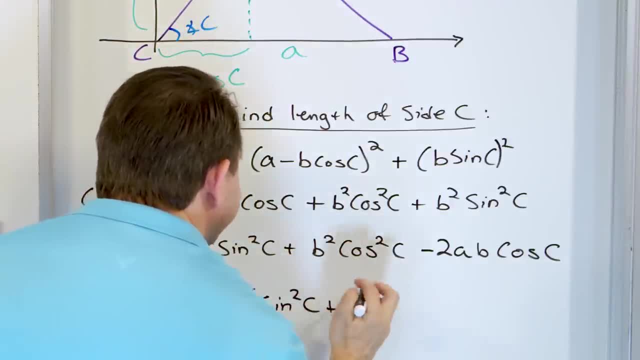 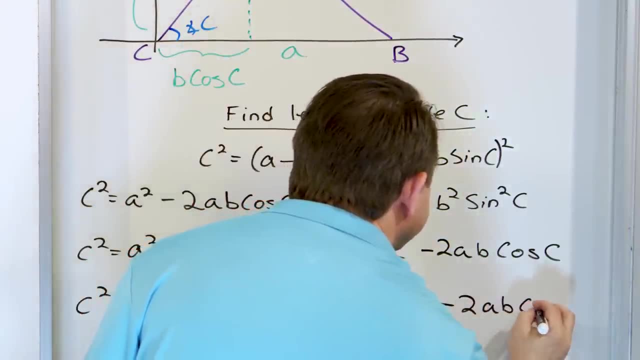 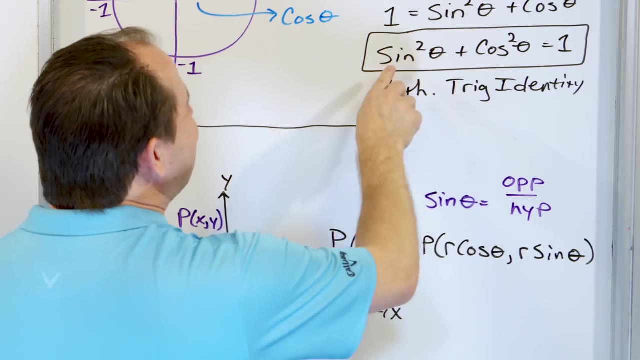 left is sine squared of the angle C cosine squared of the angle C. We have the plus sign there And then we have minus two AB cosine of C. But look what we have. We just said that for any angle, sine squared plus cosine squared of the same angle is equal to one. 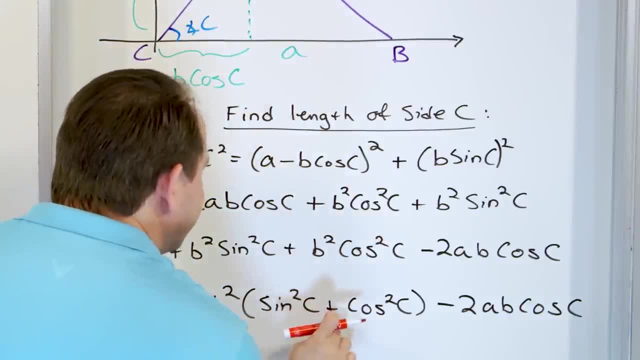 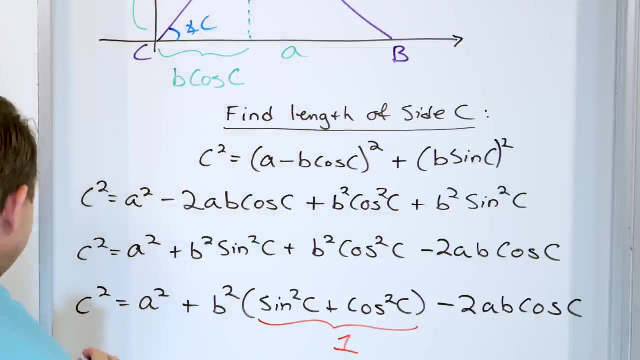 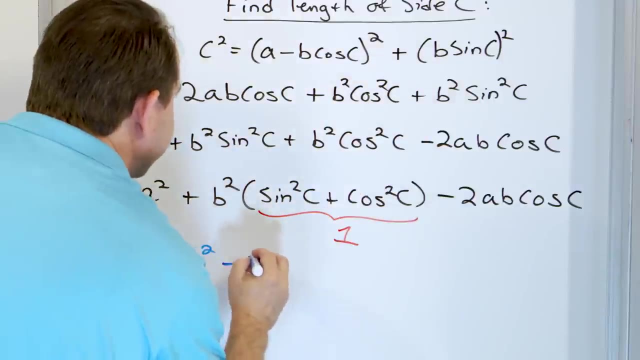 for any angle. And here we have sine squared of the angle C plus cosine squared of the angle C, So this whole term just goes to one. So what do we have left? We have: C squared is equal to A squared, plus this B squared times one. So it all disappears Minus two times A times B times the. 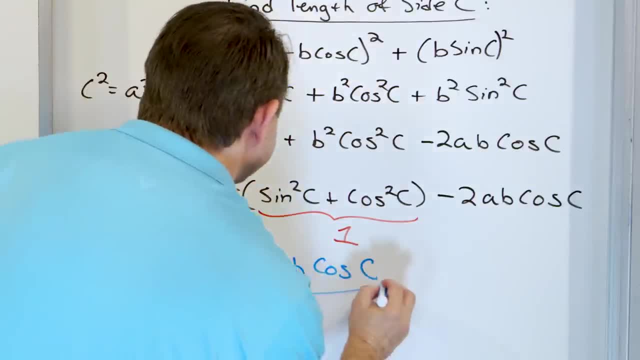 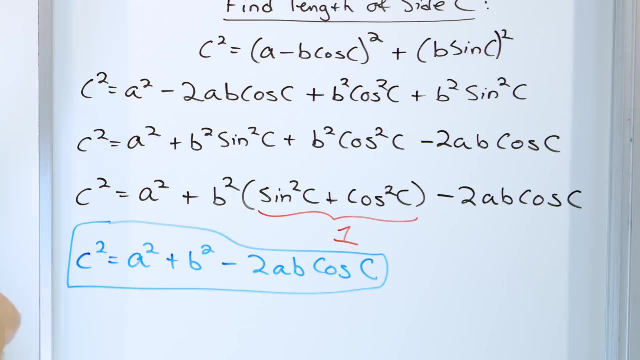 cosine of the included angle C, And this is the famous law of cosines. So two, I'm sorry, C is C squared is A squared plus B squared minus two AB cosine C. So from the top general triangle, no 90 degree angles. here is a point up, here Let's find 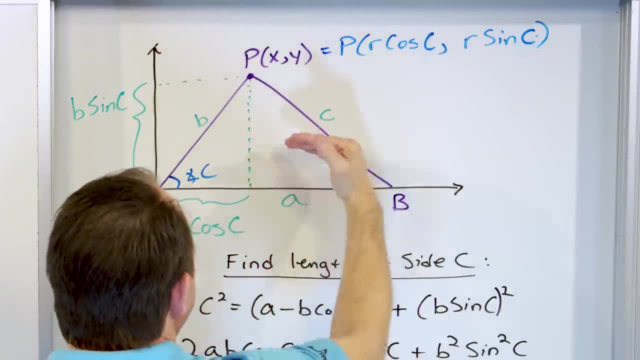 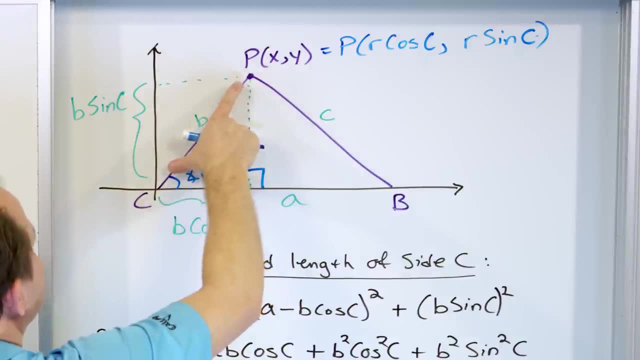 the distance C. So C squared is the other two sides of the right triangle. This is a right triangle squared, So this side is squared, but this side- we just said we can write it as this side- B- times the sine of this angle C, So this becomes squared. That's where that. 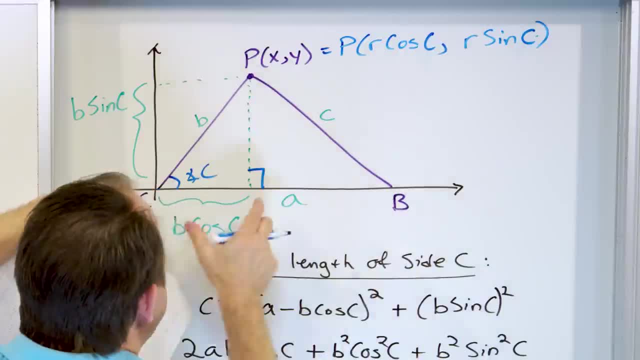 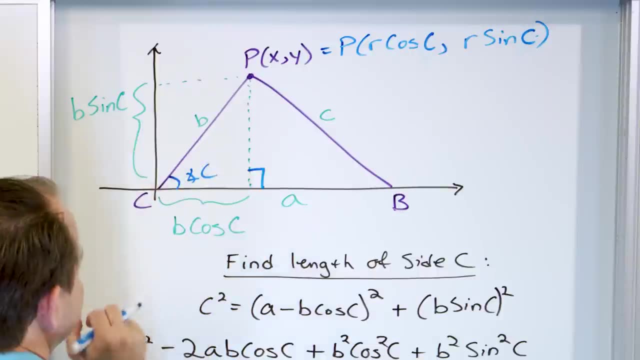 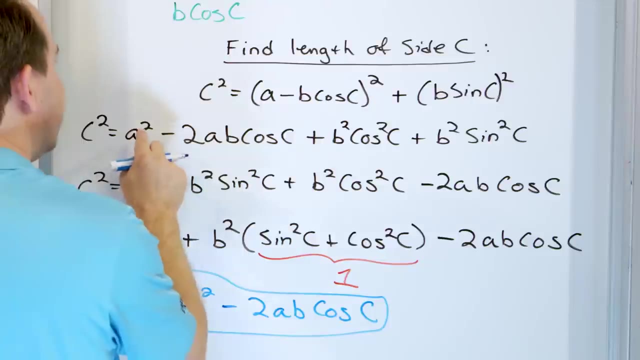 is This side squared? Is the whole side squared minus this little part, A minus, and this was B cosine of this angle C here. So that's what that side is there. So this entire subtraction is what this little side is and we have to square it. Then we do kind of foil on it. So this squared minus two times A times. 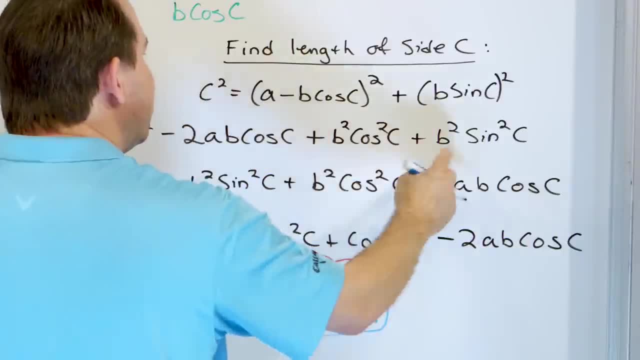 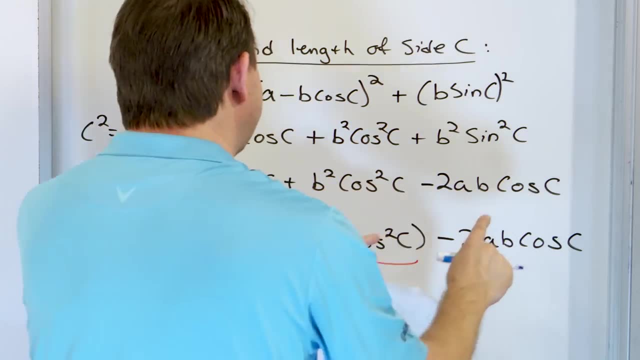 this thing here And then we squared the last term. Then we just regroup these two terms together. That's all we did is kind of rewrite the order and bring them here And then this one we brought in. Then when we factor out, we see that this is one and it all falls away And the only 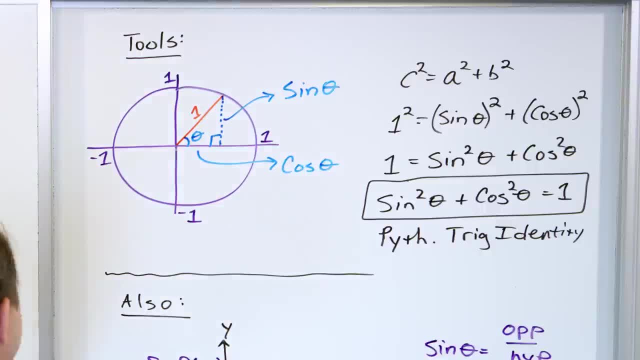 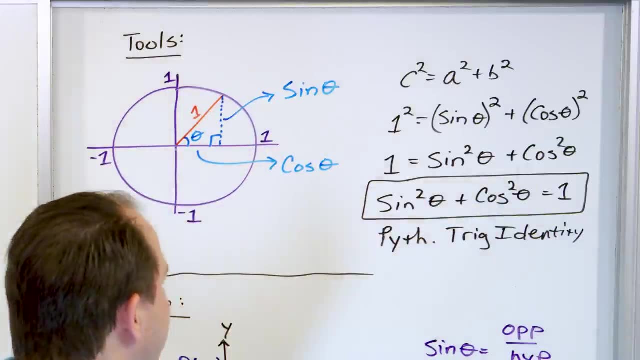 thing that you really need to understand. that is that two pieces of information: When you draw a unit circle, sine squared of any angle plus cosine squared of any angle is one. We went over that. And then the other thing is that in the xy plane, any point you can write,